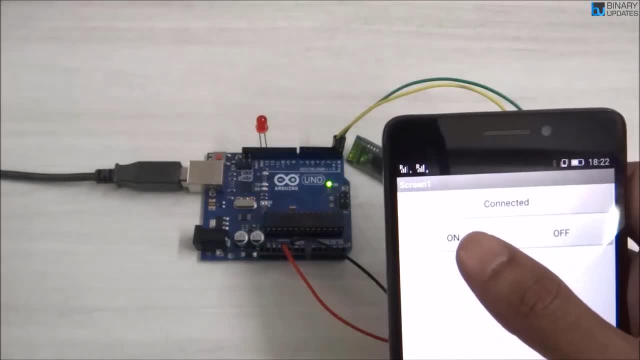 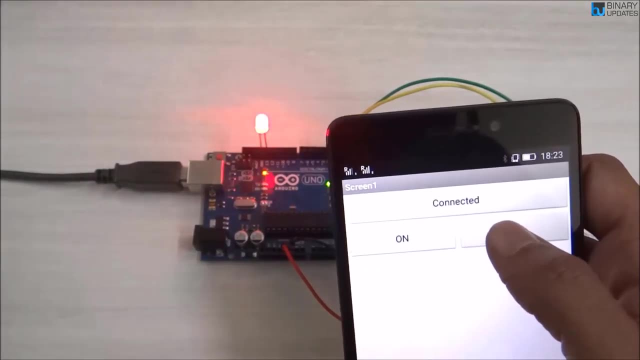 So in this lesson we will going to learn how to control the led connected to arduino uno using bluetooth app, right? so you see here, i press the button and led turns on, and i press the off button and led turns off. right? so here what we have is hc05 bluetooth module. 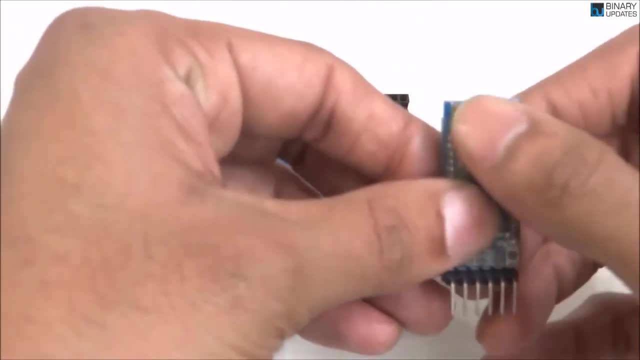 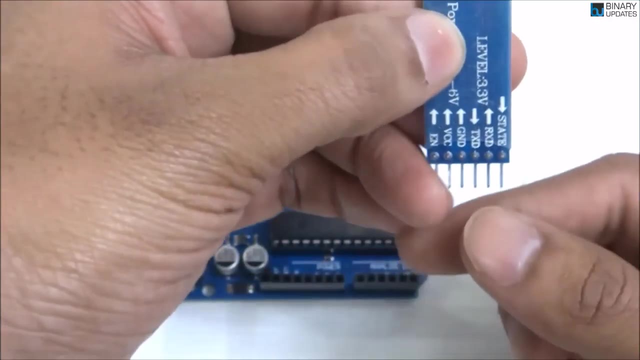 if you look at the front side, it will look like this: it will show you some kind of antenna here on hc05 bluetooth module and in the back side, when we look at that, we will see the every pin on this module. okay, look at this. every pin on this bluetooth module has a name. so say: 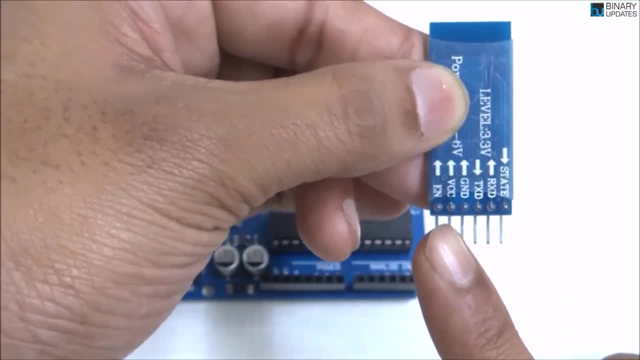 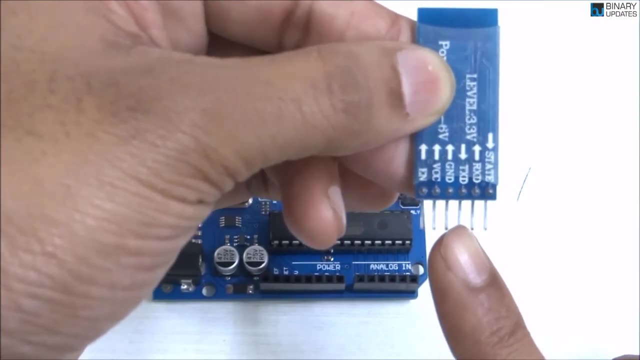 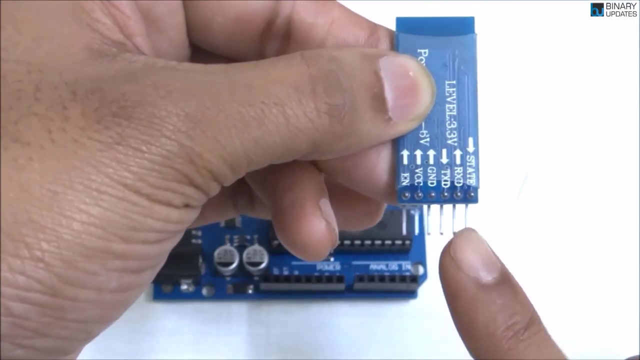 for example, the first pin is in enable, en. second pin is vcc, then this one, third one is a ground and then the fourth one is a txt. fourth one is, i think fifth one is rxt and then the state right. so this is how the the pin label has been given on this hc05 bluetooth module: like enable, vcc, ground. 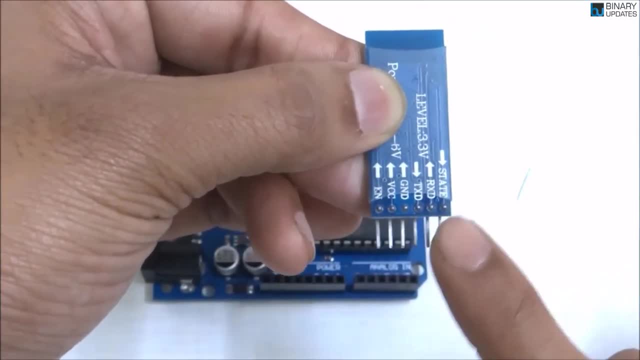 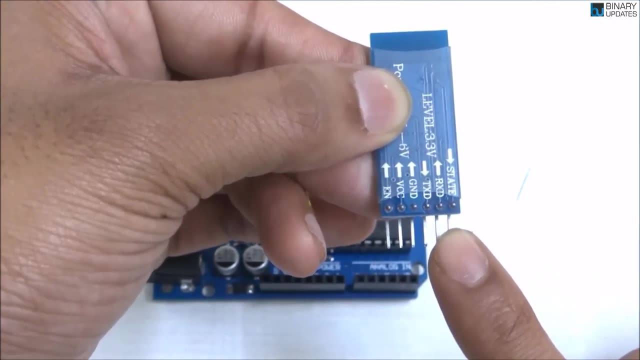 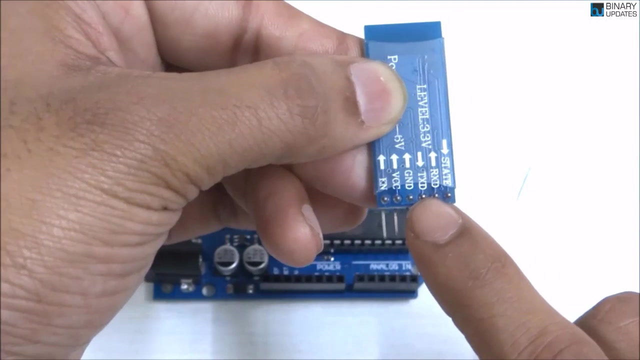 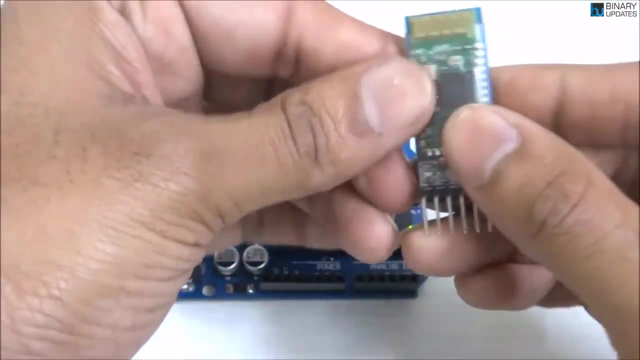 tx rx and tx state, So enable and state. these are the two pins we are not using here when it comes to connecting HC05 Bluetooth module with Raspberry Pi. and the other pins, like VCC- ground to power up- and TXRX, we will be using in order to communicate this HC05 with our Arduino Uno. okay, So let's take. 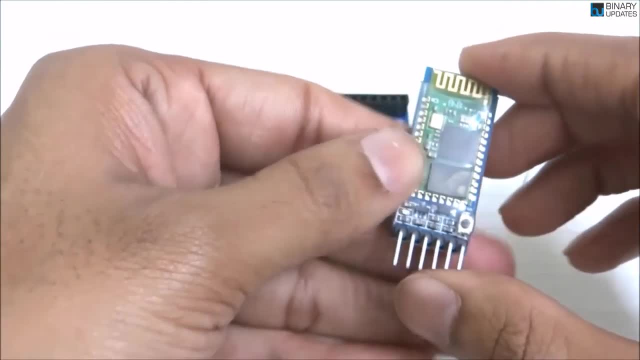 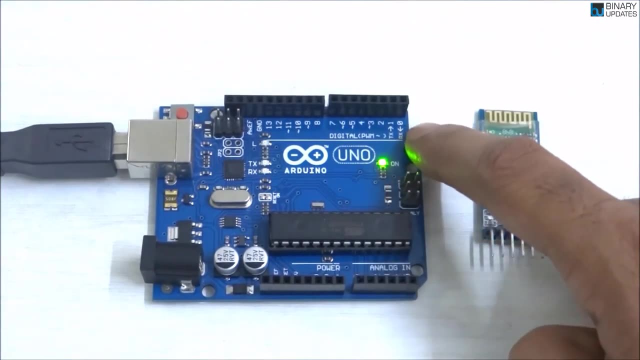 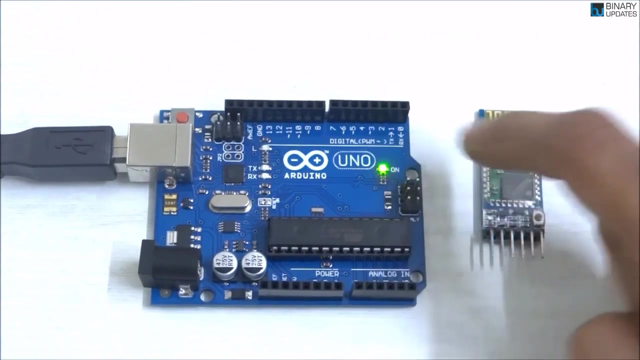 this Bluetooth module and connect it to Arduino Uno. So here we have a Bluetooth module and you see, on our Arduino Uno there are the pins, like the first pin is the RX, okay, and like digital pin zero is RX and digital pin one is a TX, right? so if you can look at this carefully, 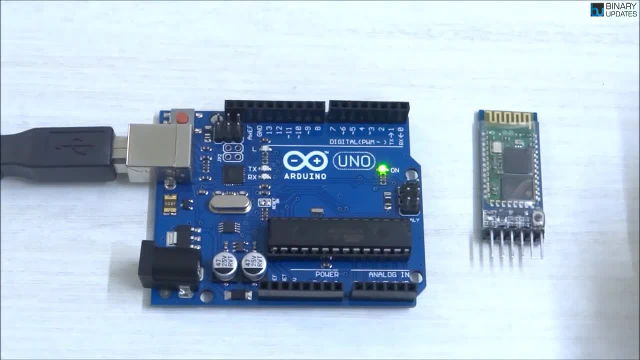 you can able to see it: pin number zero on Arduino is RX and pin number one on Arduino is a TX right. So basically, to make the communication between this HC05 and Arduino Uno, we need to have a connection between this HC05 and Arduino Uno. 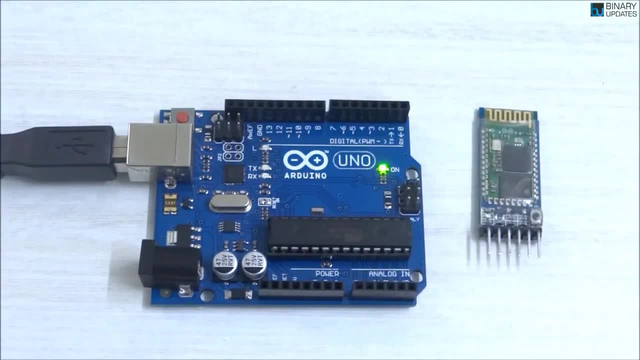 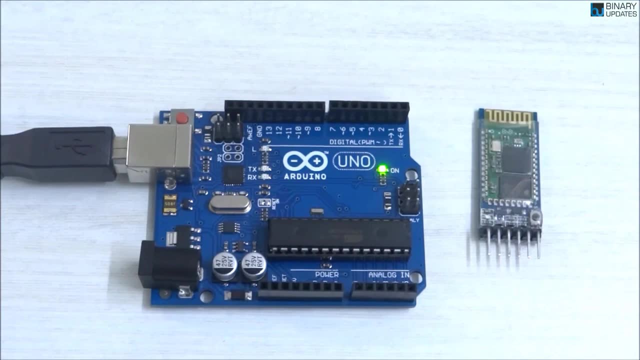 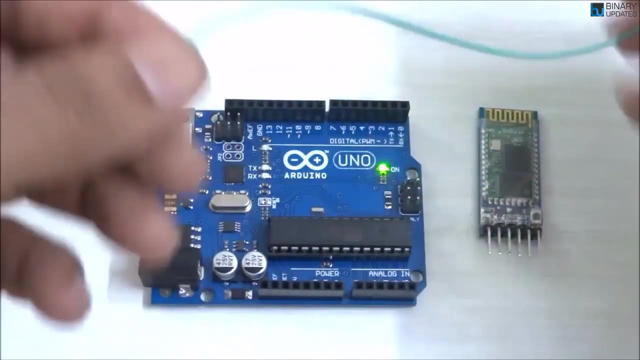 We need to have a couple of male to female jumper wires, right? so we can take the jumper wires and start connecting this HC05 Bluetooth module with Arduino Uno, right? So let's take the first male to female jumper wires and let me take the back side of the. 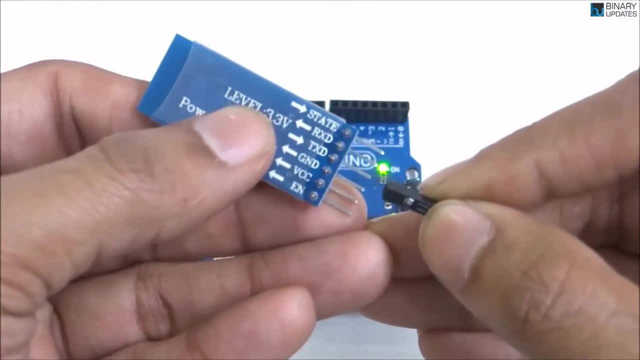 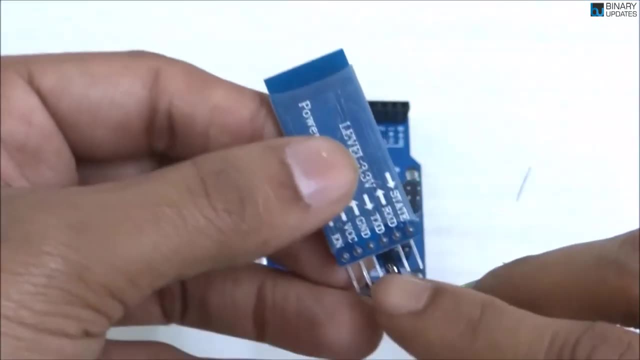 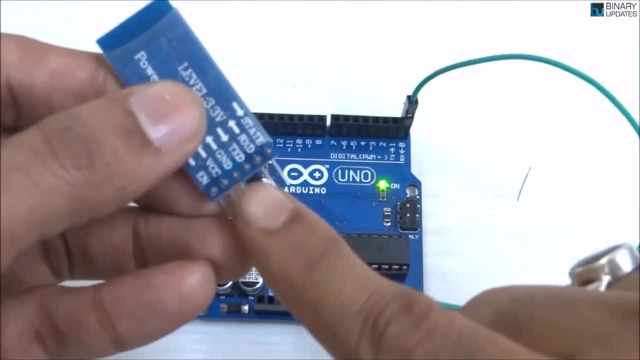 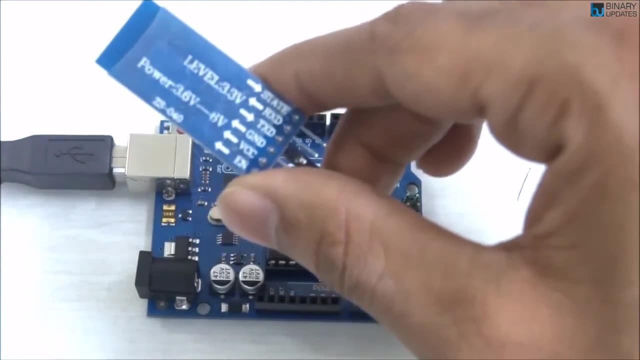 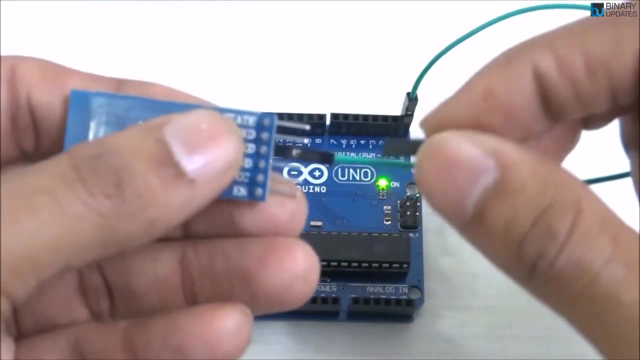 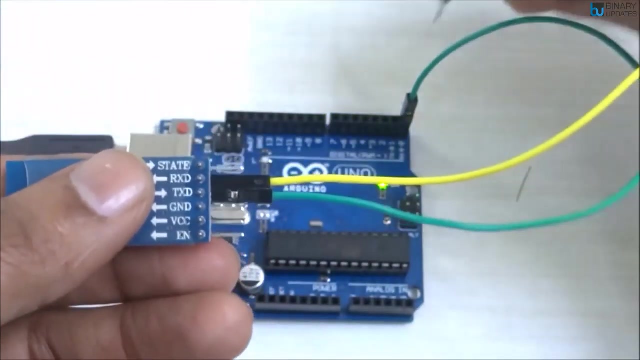 okay, because it's a transceiver, the TX on Bluetooth module. go to RX on the Arduino Uno, right. Then take another jumper wire- okay, male to female jumper wire and the female part of the cable we're going to connect to the RX. okay, and then this yellow color RX, we're going to connect to the TX on Arduino Uno. 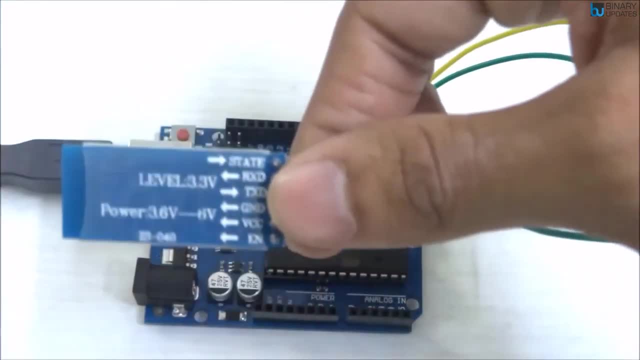 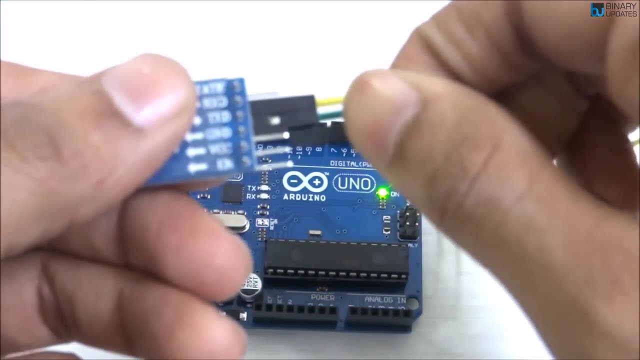 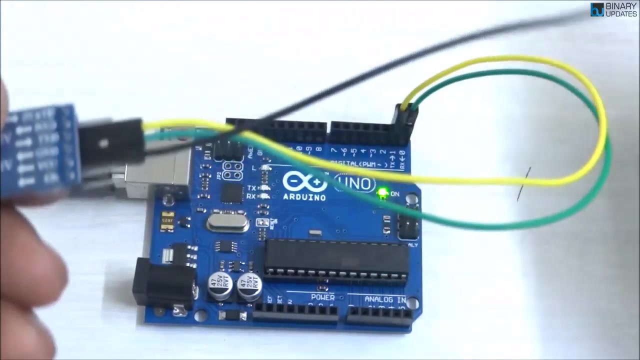 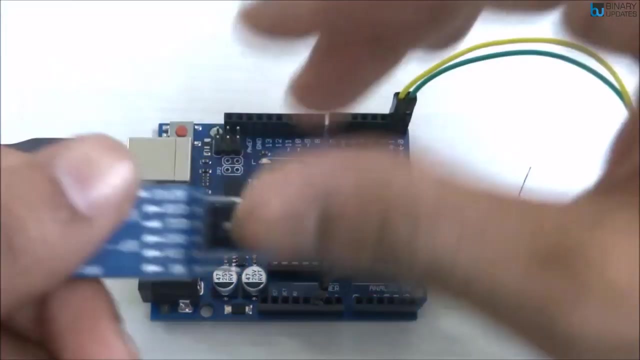 right, so that's how it's going to connect. okay, and then we will take one black color and we should connect the ground on HC05 to the ground on Arduino Uno. I would rather use this one, okay, ground pin on Arduino Uno. okay, and then only one remains, which is the. 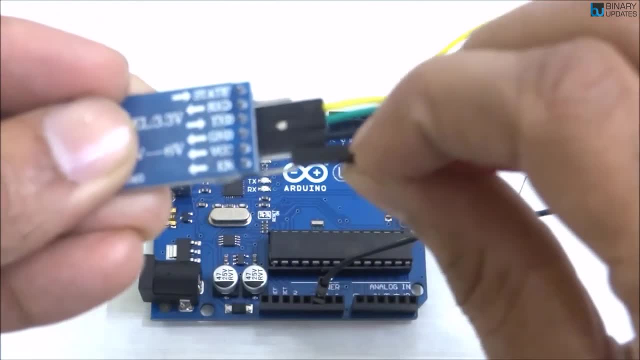 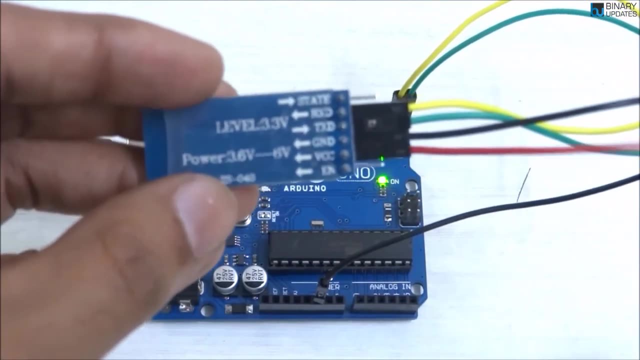 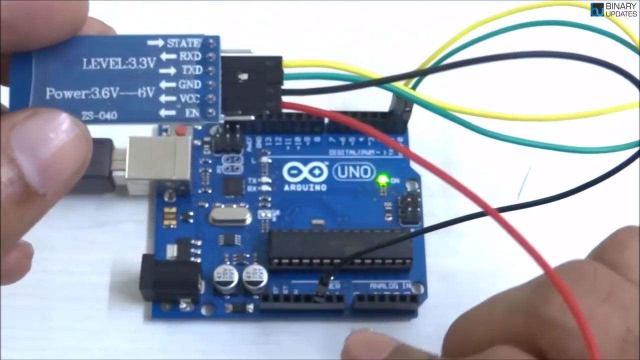 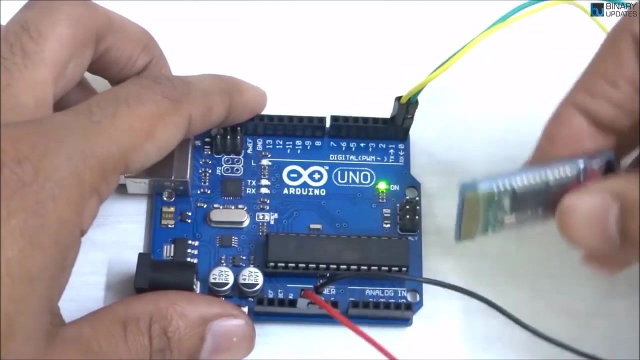 VCC. so here is a VCC pin, okay, and that will connect. to look at this, it says like 3.6 to 6 volt, right, so I would going to connect to the 5 volt on Arduino Uno. okay, and this is how we will have to connect HC05 Bluetooth module with Arduino Uno. 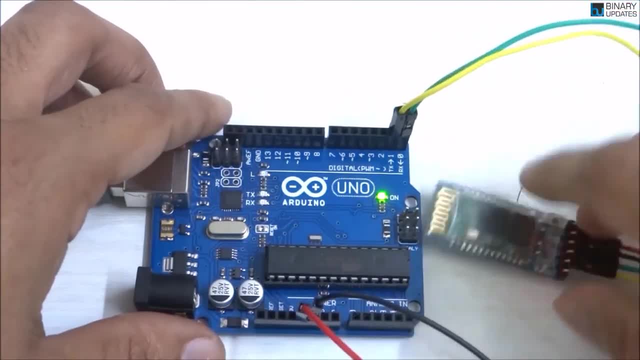 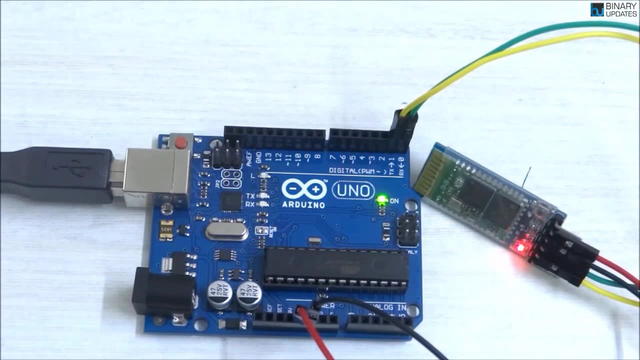 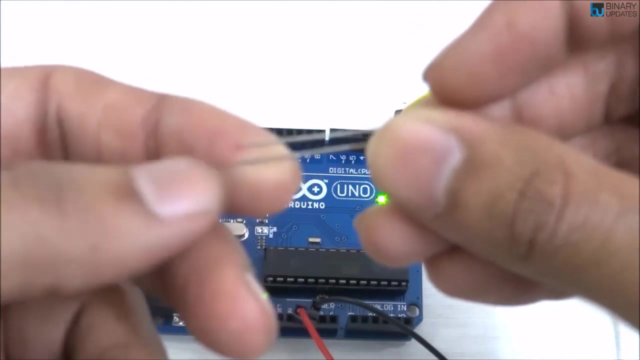 okay. so I don't know it's not staying here, but I think it looks a little bit better now. and then we can take one LED. the longer leg of the LED will going to connect to 13 and the shorter leg of the LED will going to connect to 13.. 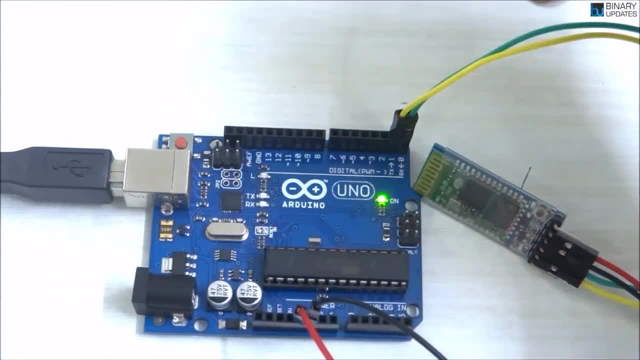 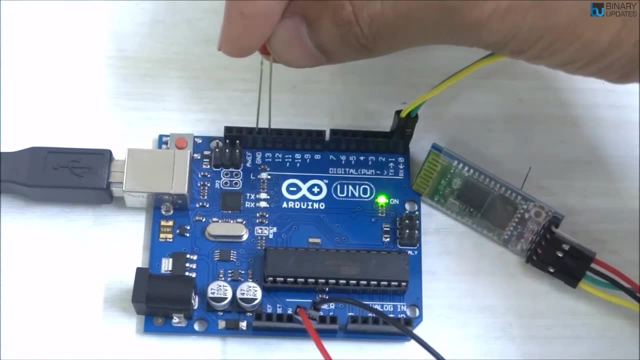 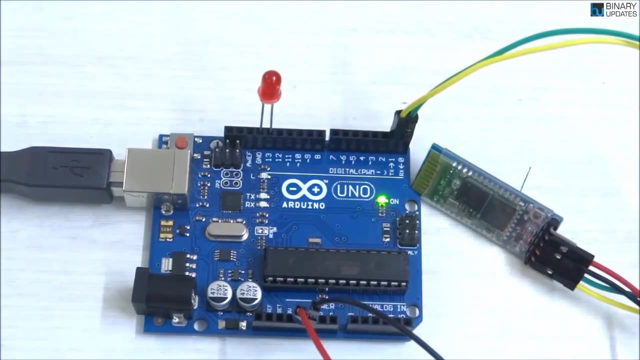 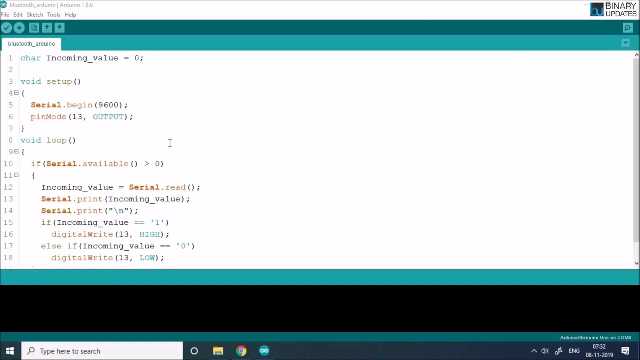 to the ground, according to the program that we have written right. So I will take this LED, and longer leg is to 13 and the shorter leg is to ground. Let me just plug in. Okay, So this is how you will going to connect HC05 Bluetooth module with Arduino Uno. So, basically, 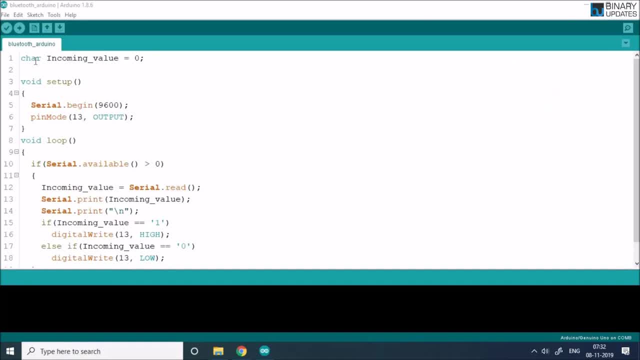 this is a piece of code that we want to upload on Arduino Uno. What you see here is a character variable. We have to define a character variable- incoming value, and we make it as a zero right in the beginning and then in a set of function. you see, every Arduino program has to have. 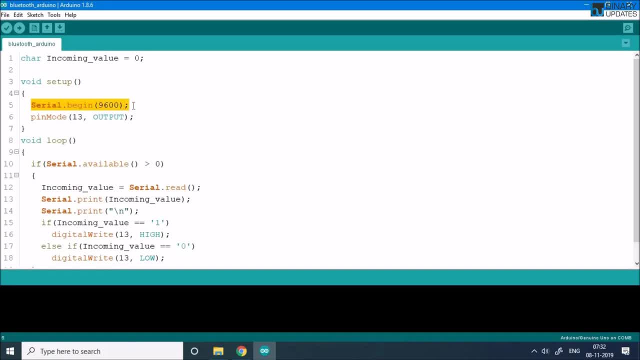 a set of function. We have to say serialbegin 9600, because we will be connecting this HC05 to Arduino Uno over DX and RX pin, which is a serial UART communication protocol, and that's why we also have to initialize this serial UART in order to receive the data coming from mobile. 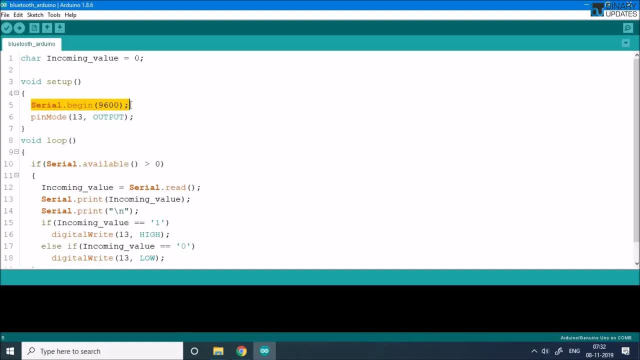 app to Arduino Uno and that's why we say serialbegin 9600, port right, and then our LED is connected to pin number 13 on Arduino Uno. That's why we say pin mode 13, comma output, to configure pin number 13 on Arduino as an output, configure into the output mode basically. Then in the 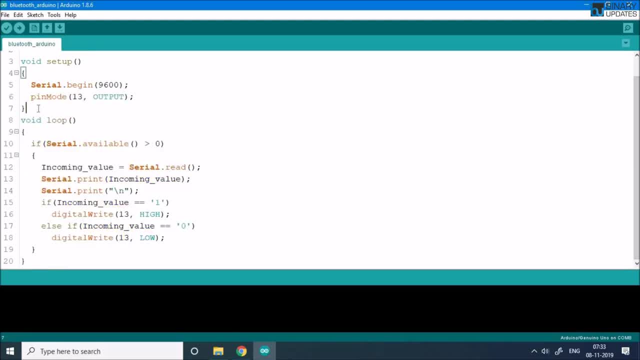 loop function. Here is a loop function. Okay, let me make it a little bit readable here. Okay, in the loop function, here comes the logic. So this is the logic. this if statements basically takes care what to do when you press the button right. So look at this. if serialavailable, so when you press the button on your mobile. 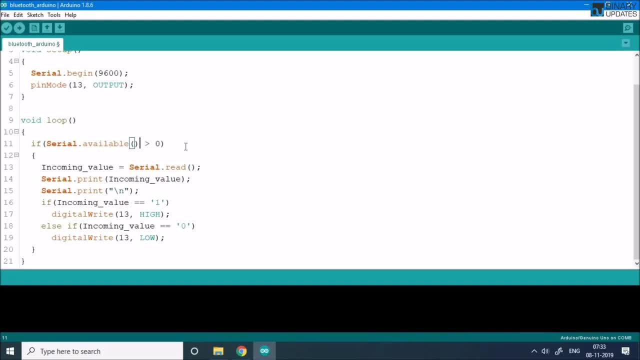 app the on button which we will going to create later on this. when we press the on button, then it will send one character one, or maybe the number one, to our HC05 Bluetooth module which is connected to Arduino. So when Arduino receives one, okay means basically. 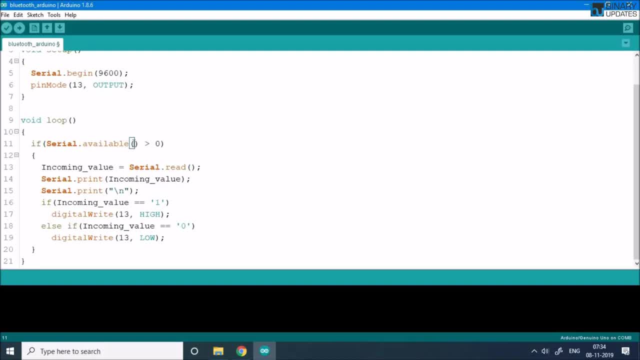 when HC05 receives something means a serialavailable. if one comes, that means there is a data available. If it's greater than zero, that means the data is available. If data is available, then we want to Say serial dot read. we read the data and store into incoming value variable right. 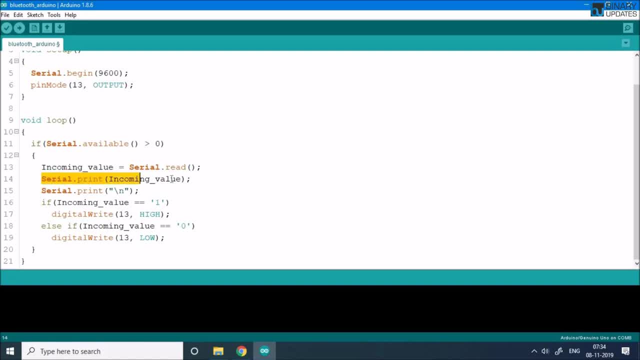 And then we want to print this incoming value variable by saying serial dot: print incoming value and then just give you know new line. So it will just every time whenever you press the button, the new value one and zero will come on a new line, right, And then we check. 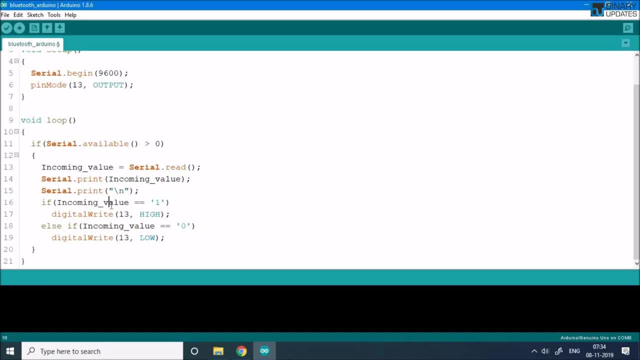 here with the EPL statement. Okay, So if incoming value is one, then it will turn on the LED connected to pin number 13 and then we say digital right, 13 comma high. So this will turn on the LED. So basically, when we press the button on on our mobile app, it will send one from the mobile app. 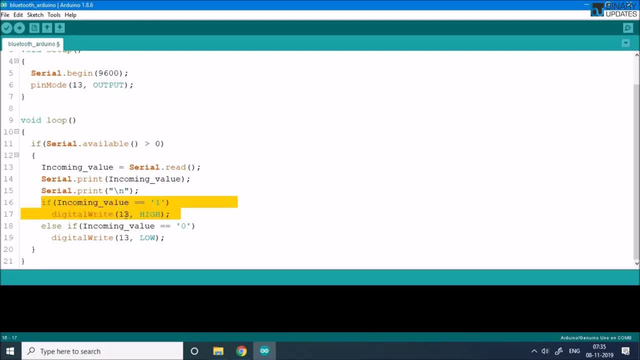 and it will turn on the LED connected to Arduino, pin number 13.. Right, so it will turn on. So when you press the off button on the mobile app, it will send a zero. mobile app will send a zero To the CDL at zero five Bluetooth module and Arduino. and when Arduino receives the 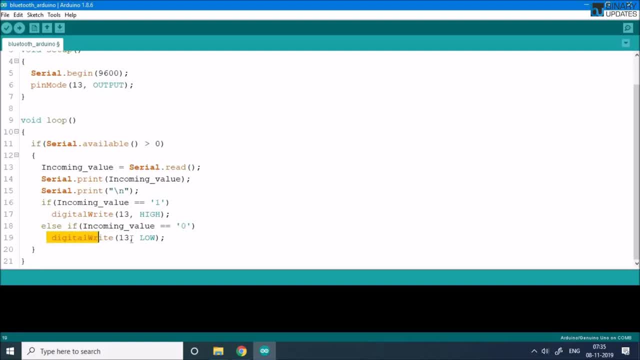 value zero after pressing off button, then it will turn off the LED connected to pin number 13.. And that's why we say digital right, 13 comma low. Now, if you're not aware of this code, if you have a problem, then you might want to check out my serial communication. 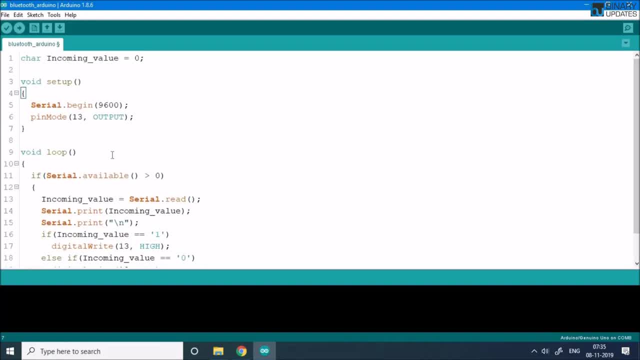 with Arduino Uno tutorial and then you will be good to go with right. but I believe it's not very difficult. It's just like we are just reading a serial data and then see if it's one, then turn on the LED connected to 13. if it's a zero, okay, then turn off the. 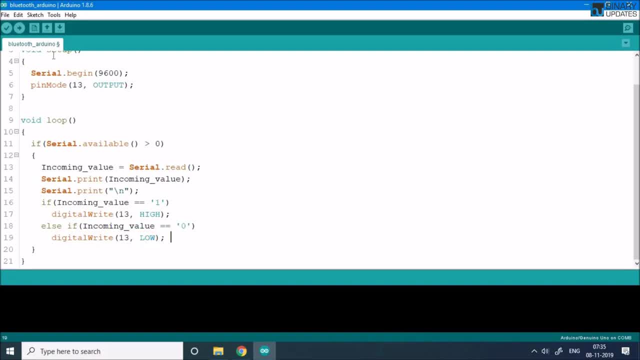 LED connected to pin number 13 on Arduino Uno. The next step is we have to go to tools, make sure the board Arduino Uno is selected, go to tools once again, go to port and select the COM port where your Arduino Uno is connected And then upper left corner there is upload. 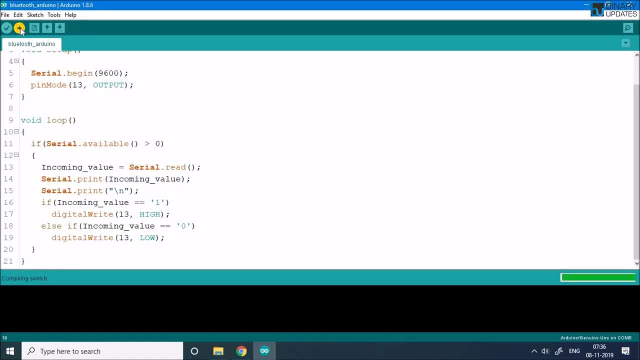 button so we can click on this upload button And this will upload the code on our Arduino Uno. And after uploading the code, then only we have to connect hc05.. So make sure those things very, very important. if you have connected this hc05 module with Arduino Uno, then you will not see. look at this in lower left corner. 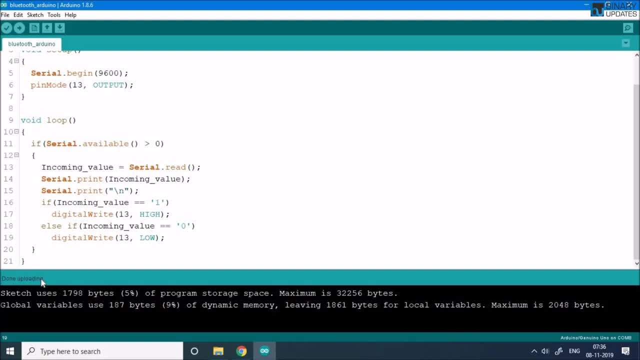 done uploading. you can't able to upload the code because the uploading process of the code also uses dxml. So first upload the code on Arduino Uno and then connect hc05 Bluetooth module. So once the code is uploaded, okay, done uploading. Now to create a mobile app using MIT App Inventor. 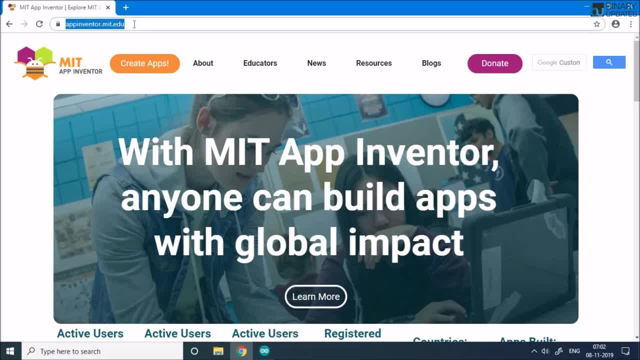 we have to browse the web page app inventormitedu, So we first have to come to this web page and then we have to click on Create Apps button here upper right corner, upper left corner. So once we click on that, it will take us to the page where 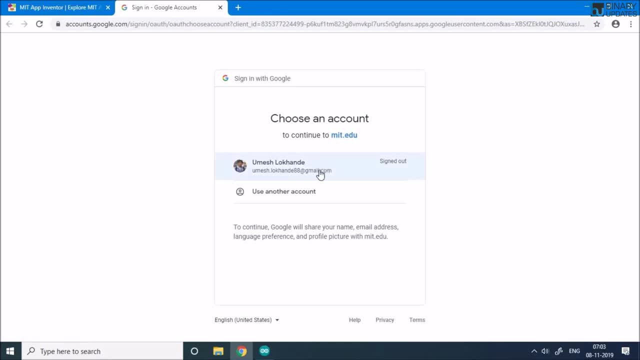 it will ask us. if you have the account, then it will not ask you. it will take you straight away to MIT App Inventor just to log in normal. If you don't have account, then I would rather like to use my Google account to associate with App Inventor, So I will click on that. 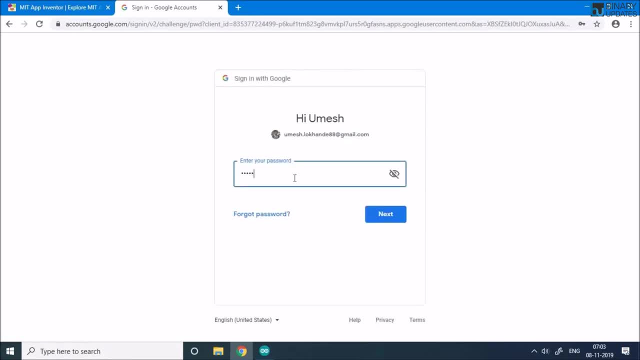 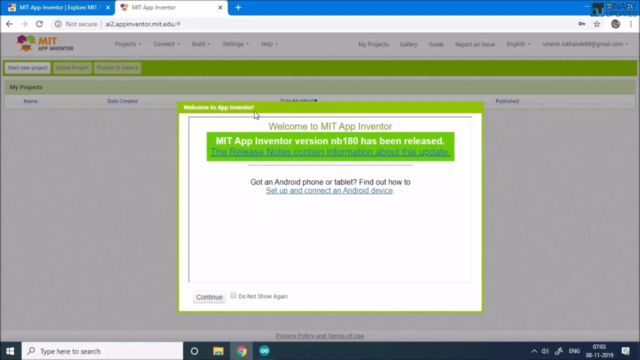 And it will create a quick account with my password. So let me insert my password here with a Google credentials And it's very easy to create account. by the way, The app inventor, and then it will take you, it will ask you: here will come to the app. 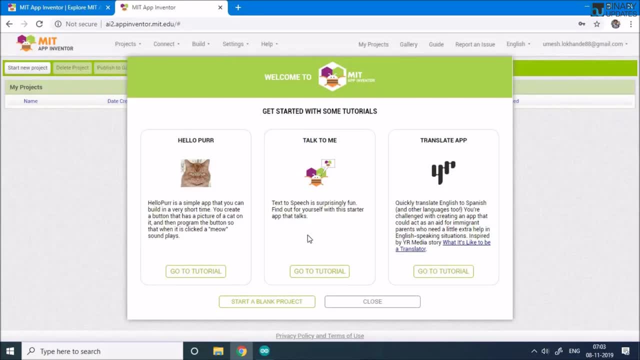 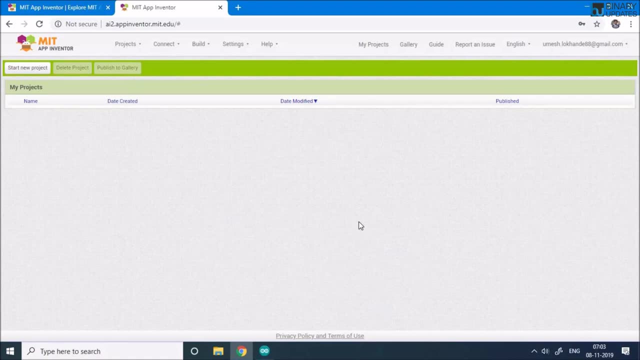 inventor and it says: like nonsense, they continue. And then here comes the another dialogue which we can say close, and here is how it looks like: right so, app inventor. So if you look at the URL, okay, it says ai2.appinventormitedu. So basically this is an app inventor to ai2. 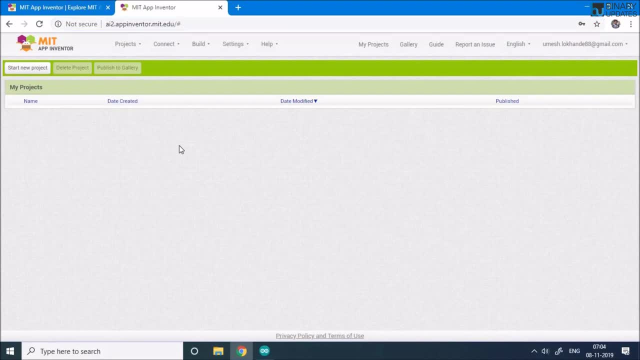 app inventor: right, Whatever you like to call now to start creating a mobile app, we have to create a project and you see there is a button called start new project, upper left corner, And I would like to give the name to the app as a Bluetooth, Okay, and then hit on okay, So you see it. 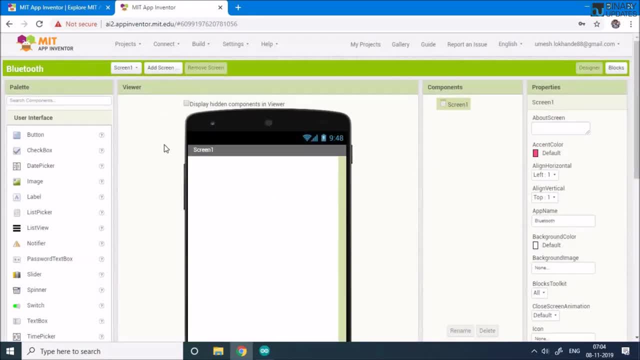 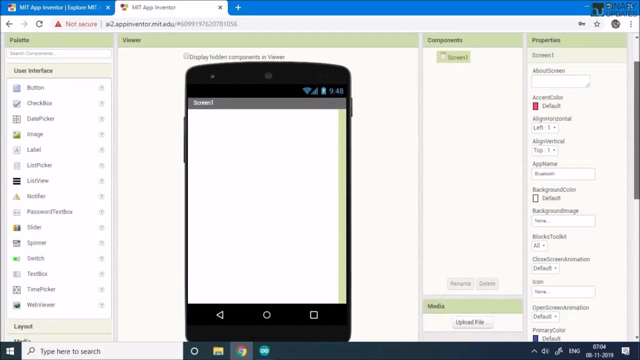 creates a project with the name Bluetooth. It takes a couple of minutes. it will straightaway take you to the project itself and you can see right now. look at this Bluetooth project which you just have created and it will present you this kind of view. right, and if you look at the app inventor, how it works is: 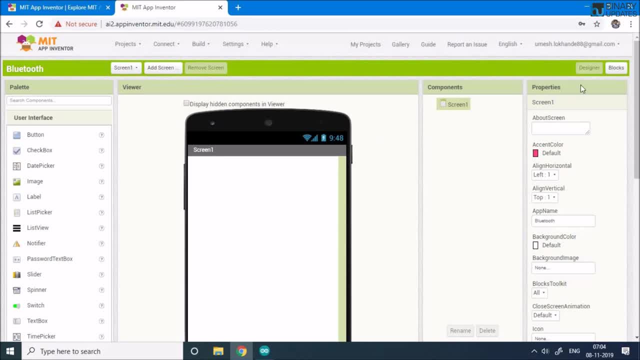 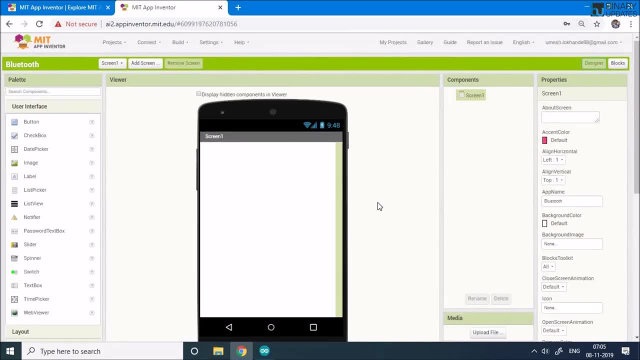 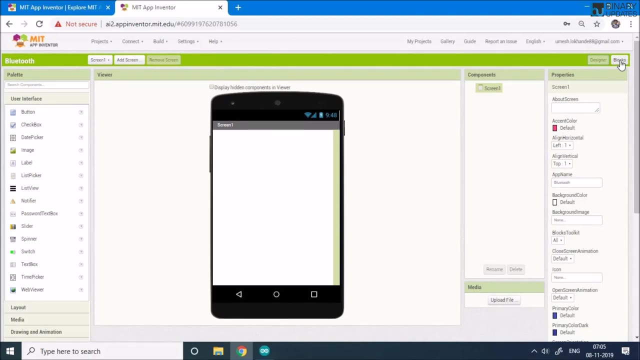 it basically gives you two views, right? if you look at upper right corner, there is a designer view which we can see. if I can zoom out a little bit, okay, just for you to see. okay, you see. so upper left corner, you see there is a designer view. so if I click on Block View, you can see there are some. 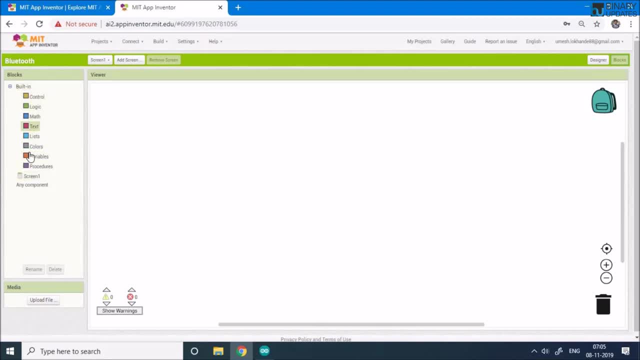 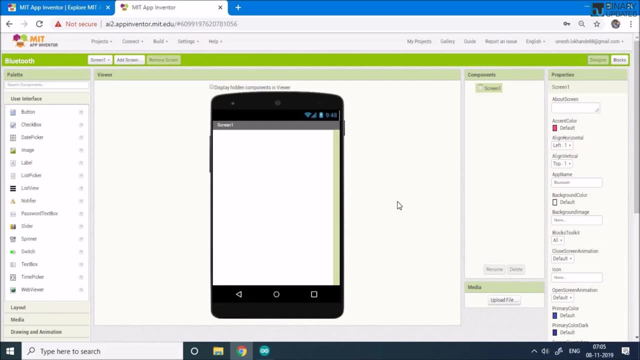 widgets in the left pan. so there we can select some widgets and then we can create an app. so designer view and the block view: okay, so we have to stay at the designer view itself and I can zoom in again so we can see how it looks like. 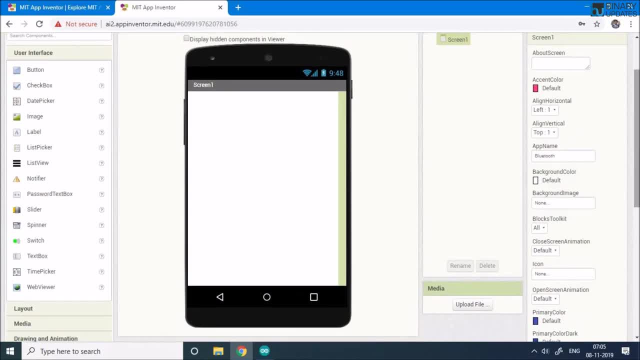 basically, and now we can start laying down the components which we need in order to make this app work with the HC-05 Bluetooth module, right with Arduino, of course. So the first component we need is: we need a list picker. so we have to take a list picker element and you see, here is a list picker. 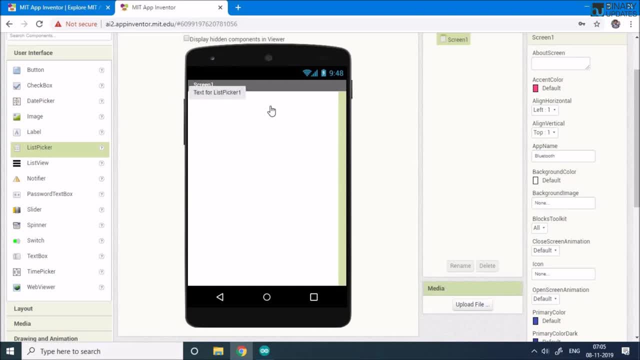 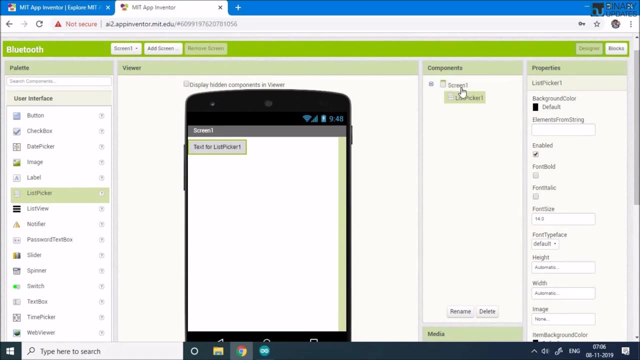 I can select the list picker in the left pan and drag it to my mobile app right. so this is a mobile screen where I can drag it down. Now I select the list picker element and you see, here is a list picker one. you see, it's added here in a component section. 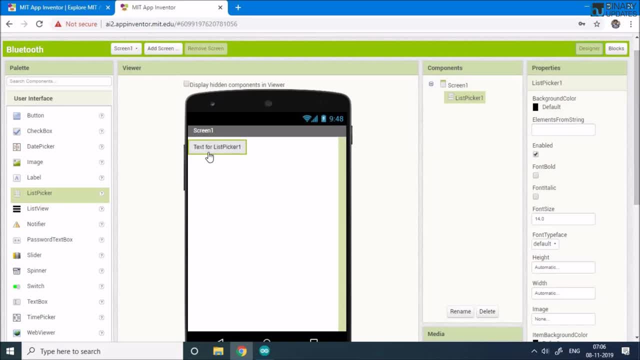 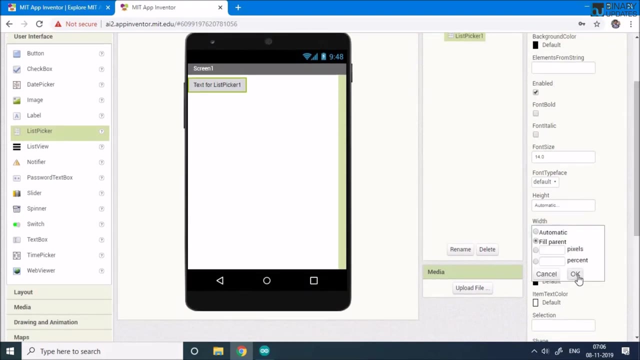 list picker one. and because it looks ugly right now, this list picker, it looks the way like it's just aligned to the left. I want to look a little bit better. this one, and you see in the left pan here the width. I will make it as a fill parent and say okay. 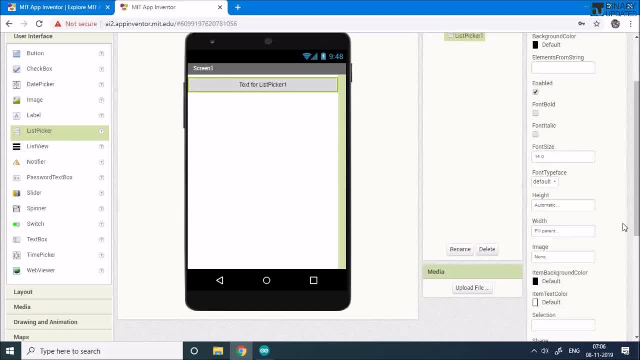 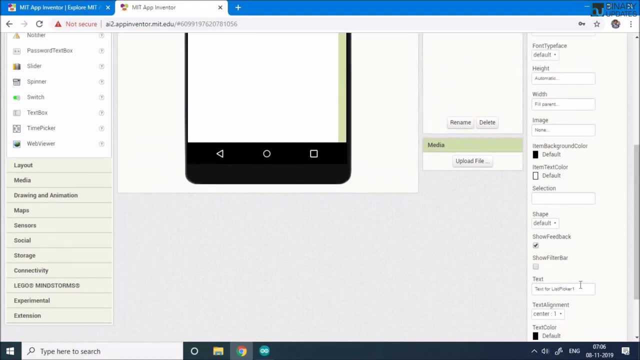 and it looks little bit better now and I would like to give it a name. so if you scroll down this, you can see there must be a text fill, right, and here is a text fill, so I would like to give the name LED Bluetooth. okay and okay. so look at this. when I 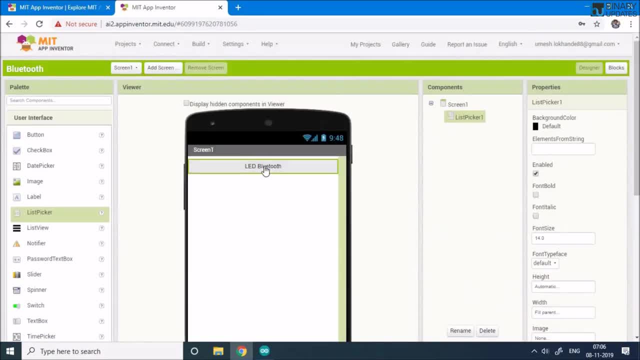 when I hit enter, you see the name of the list picker is changed. so, basically, this is a button, a normal button, which you can click, and then you will see a different Bluetooth client in a list. so there, we have to select HC05, because that's the Bluetooth module that we want to communicate with using this mobile. 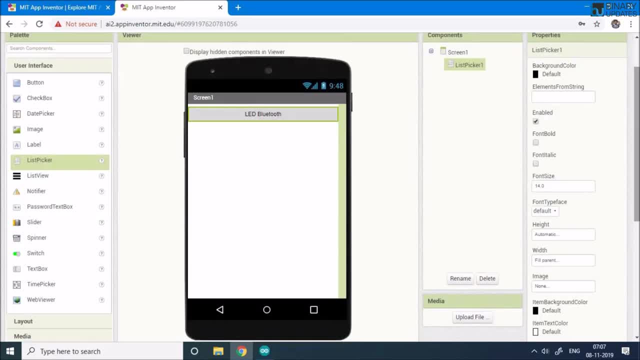 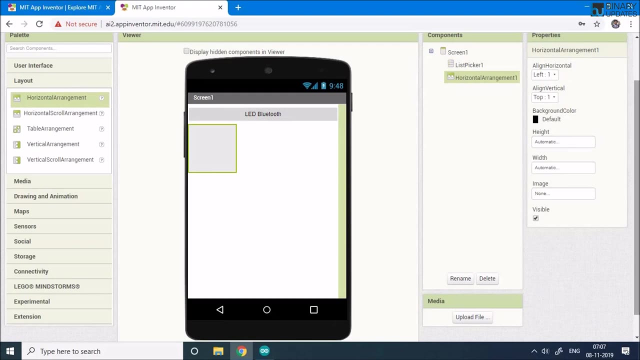 app, right, that we are creating right now. the second component we want is in horizontal arrangement, right? so if we click on layout section, there is a horizontal layout. look at this in a layout section. so I will drag it to my mobile apps and I select it, and then I would going to say width and say fill. 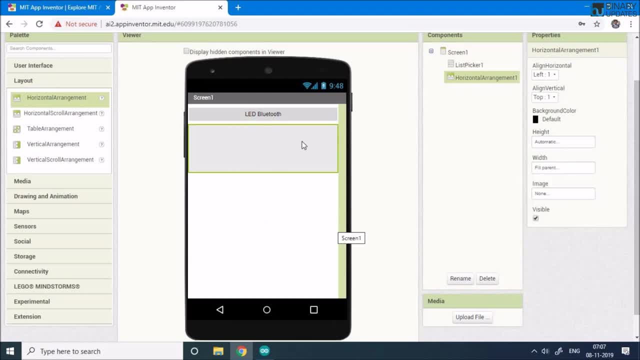 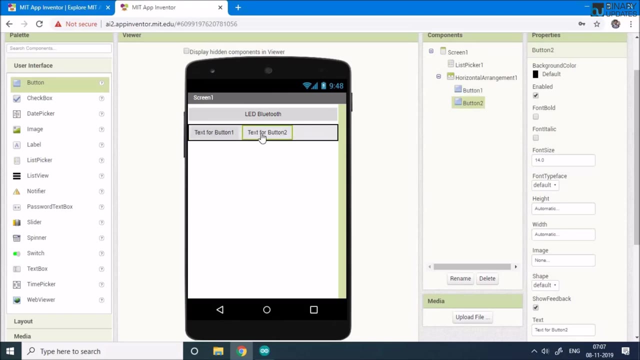 parent, and that's, that's it right? so basically that's how I will going to put the horizontal arrangement and then go to user interface once again and then select the button in the left pan and put one button, and then I will select the button and I will put another button. so now we I have two buttons right, but 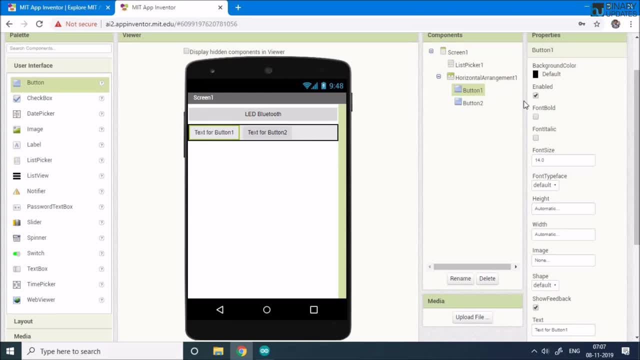 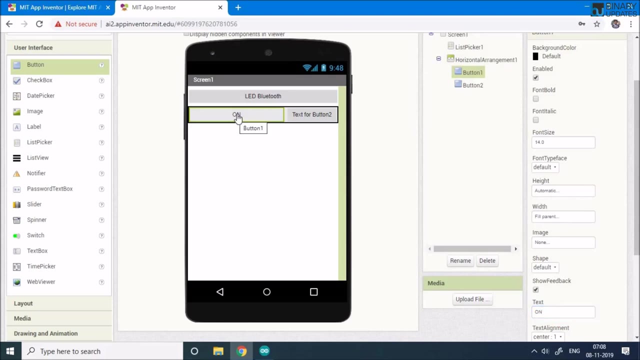 it very ugly. so i select the first button here in the user interface and i will say width, fill, parent, okay, and then again, just the way we did in the text section, i will give the name on and you see the name of a button. one is changed to on because when i want, when i press the button in 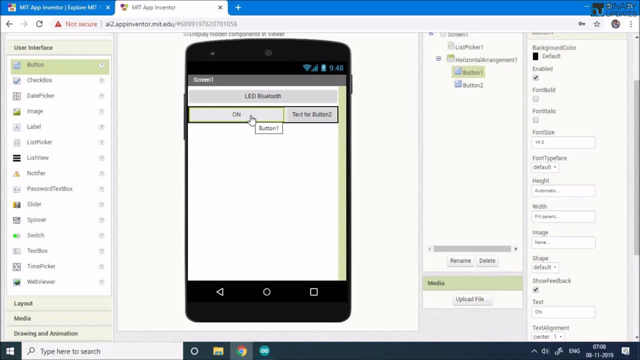 a mobile app. it will turn on the led connected to arduino using hc05 bluetooth module. and let's give it a name to other button, button number two. select the button number two and then with fill parent, hit ok, and then give it a name like off, hit, enter right. so now we have the app which 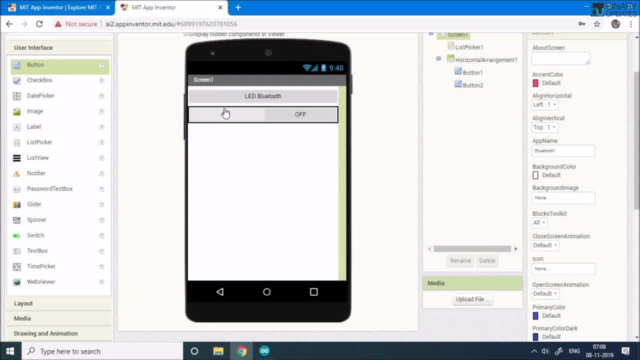 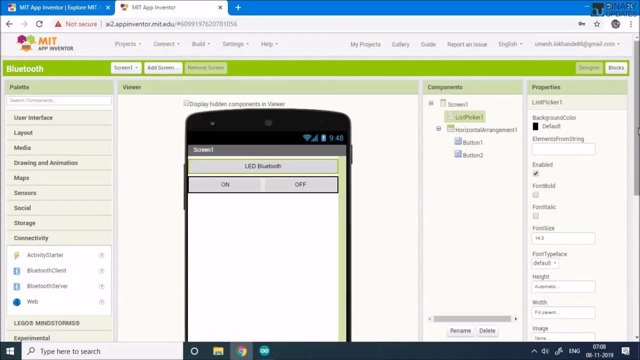 looks a little bit better and it has, um, you know, two, three, two buttons, basically, and one list picker element, right. and the one very important thing is, uh, we have to add now the button bluetooth component, right. so we will go to connectivity section, select the connectivity in left pan and select the bluetooth client from the list and then drop it to your mobile app, right. 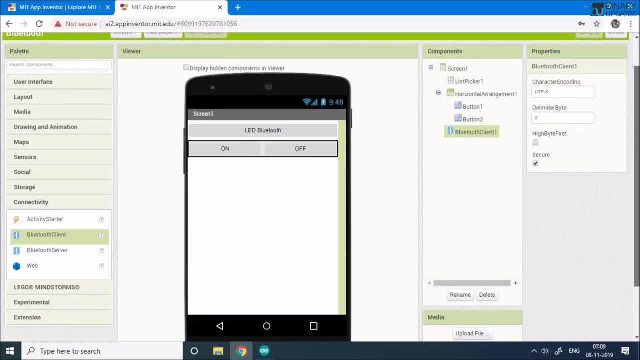 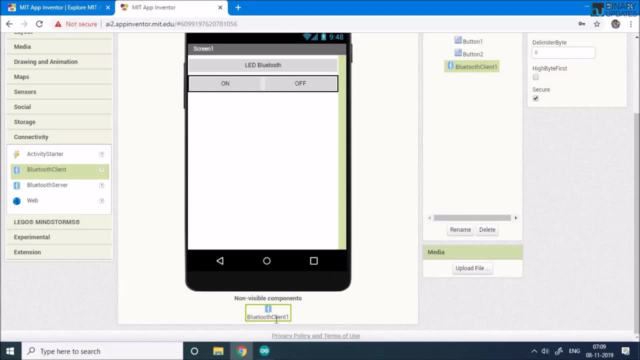 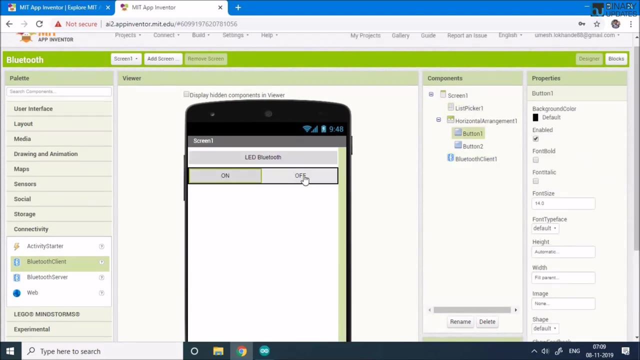 and you see this bluetooth client is added into the component list and you also see like bluetooth components will be here. it's so it's shown like bluetooth component here, right, bluetooth client one. so it will be acting as a bluetooth client. now we let down the uh user interface. 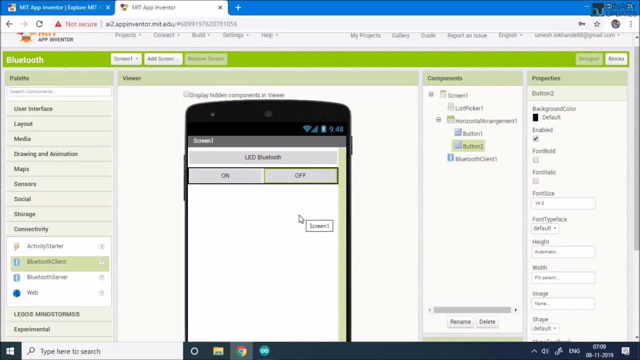 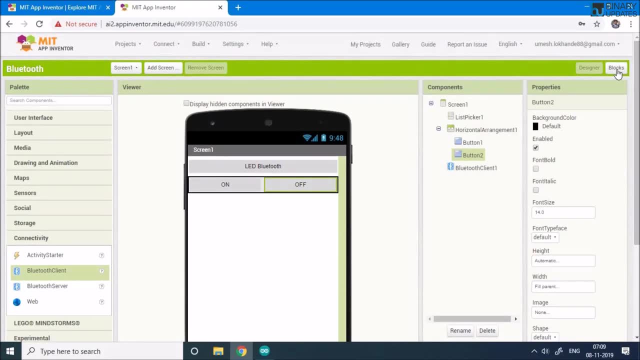 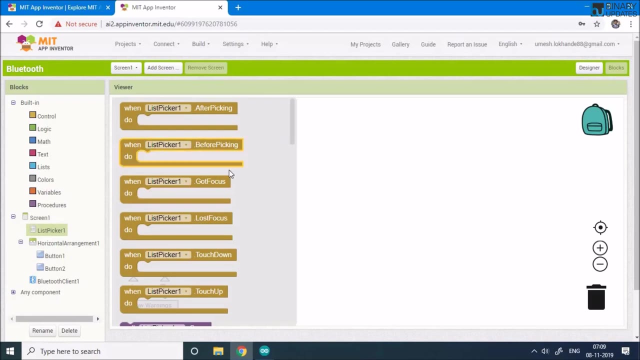 components. now we have to write a logic, um, so that, uh, it will take an action that we want it to perform through the mobile app, so we will click on upper right corner. you see, there is a block view. so we click on block view and then we select the list picker and there are two components. we 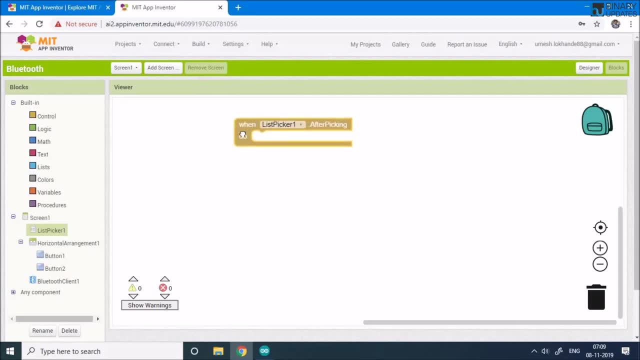 want uh list speaker, one, um, basically after picking, and list speaker uh before picking right. so, uh, before you, uh press the button, uh, this speaker button, um, and after you press the list picker, uh element, right or component, so to say so, uh, when you don't connect, then it just doesn't. 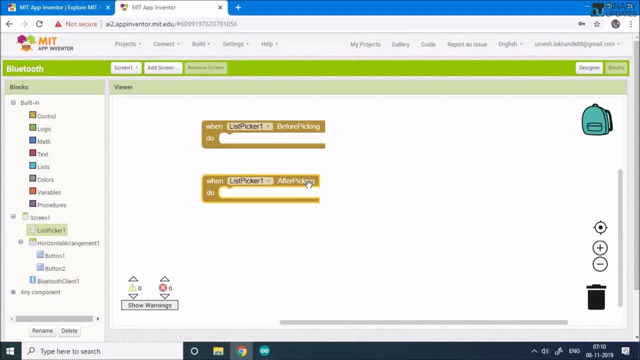 do anything, just have the bluetooth connections and when you press after picking um, okay, so when you press the button, then it will show you the list of bluetooth clients. so the next thing in order to make the logic work is we have to go to the list. speaker element again. 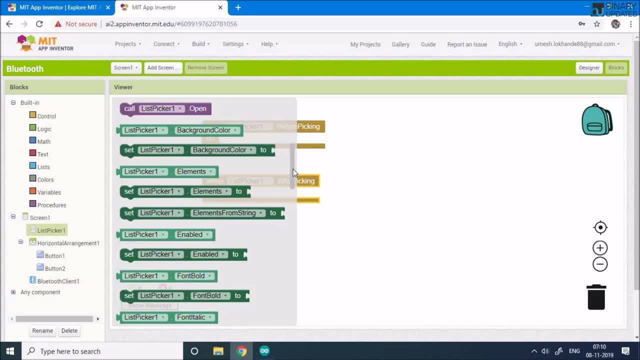 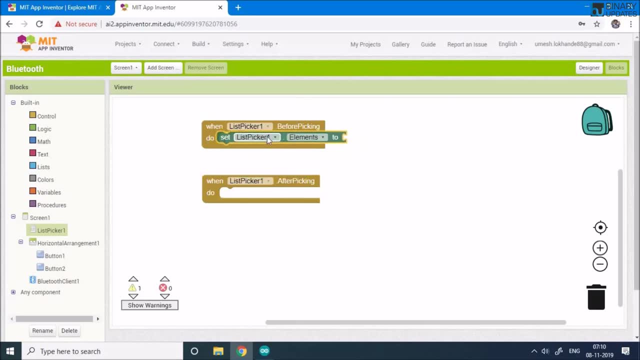 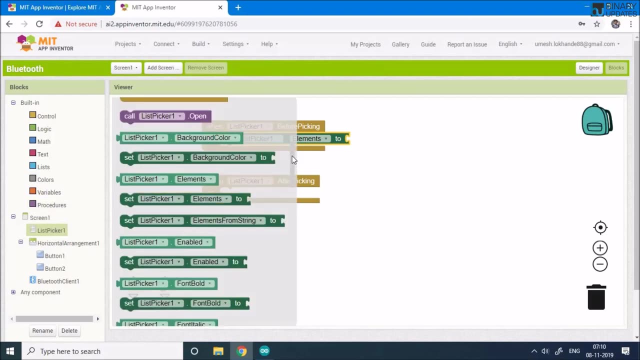 and then we have to select your list speaker, one element. so this speaker, one element that we want to put it here, just place it and it will take by itself. and then we have to use the bluetooth client, if there is any. so bluetooth client could be found into the bluetooth. 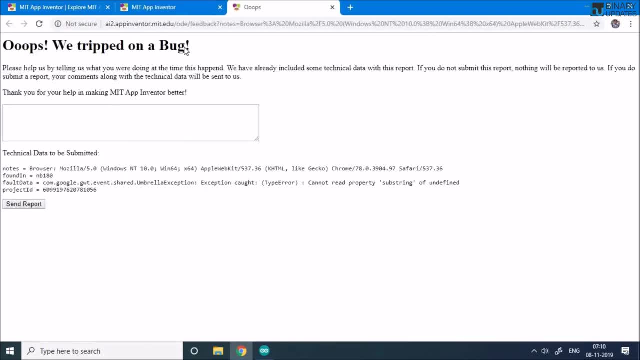 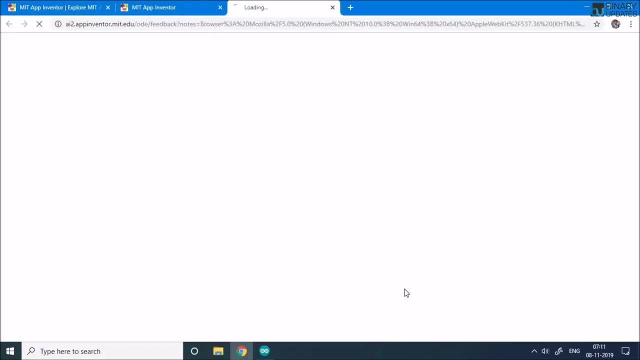 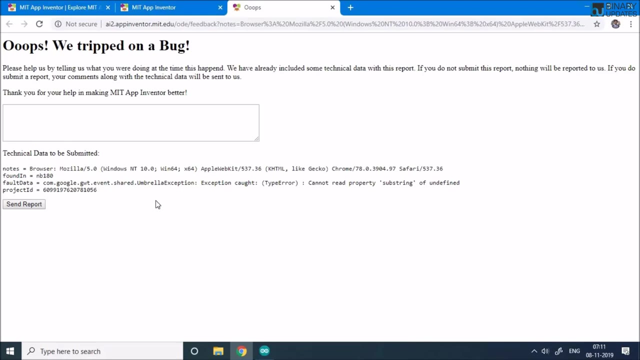 line section: okay. okay, it says some kind of issue, i don't know. let me check my internet. it's there. internet is there, right, so click on. okay. it says please help us telling what you were doing. this time happened okay, so some issue is there, but i don't mind this. rather. 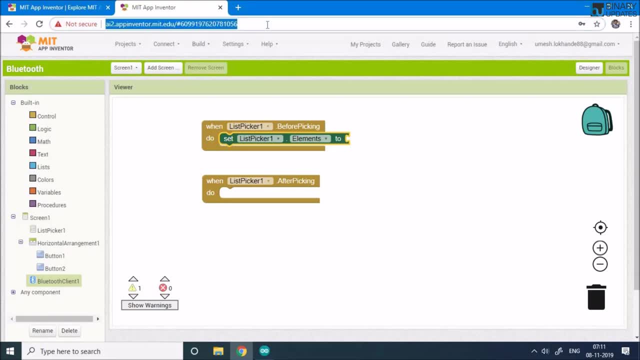 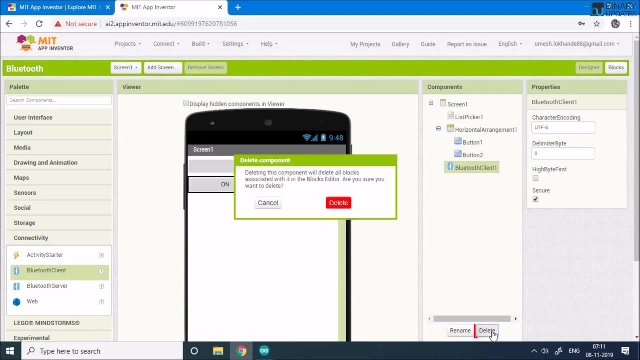 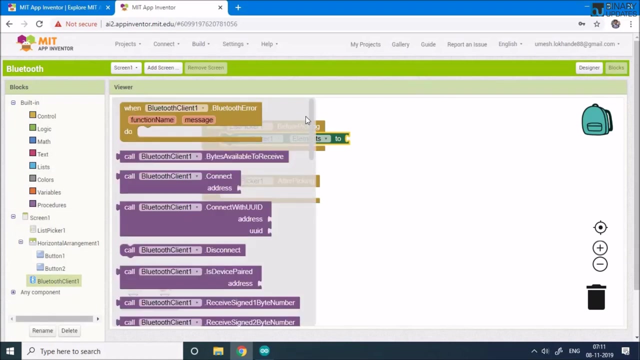 something went wrong, i guess. uh, not sure some bluetooth element is having issue. so let me go to designer view. i would rather delete this component, select the bluetooth component and remove it. okay, and now i select this and i will drag the bluetooth component once again and go to block view. and now i go to bluetooth components and now, you see, i have this. 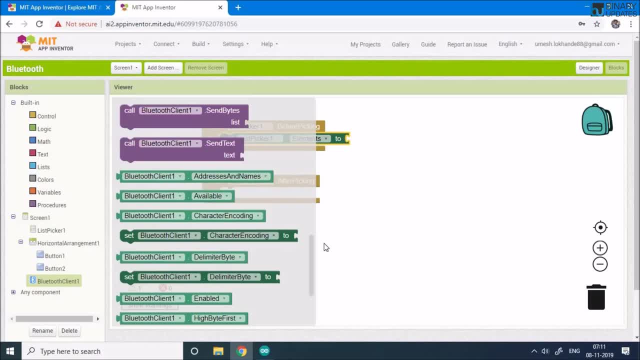 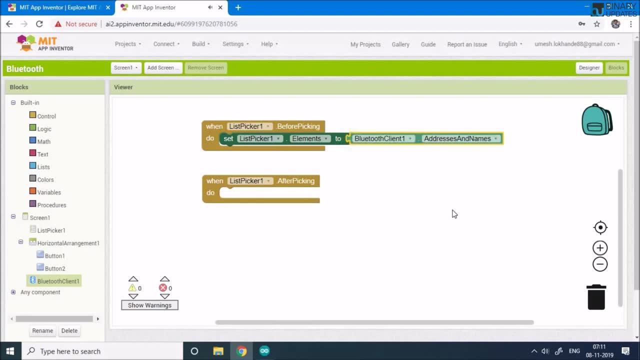 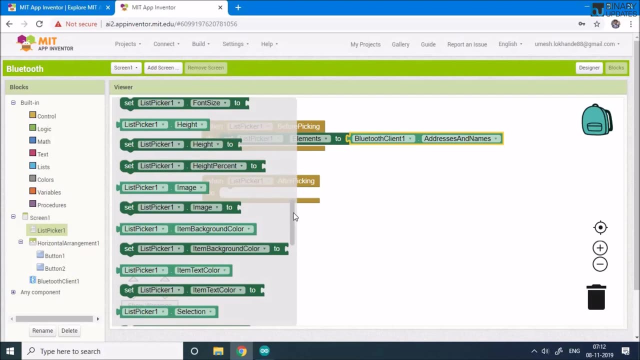 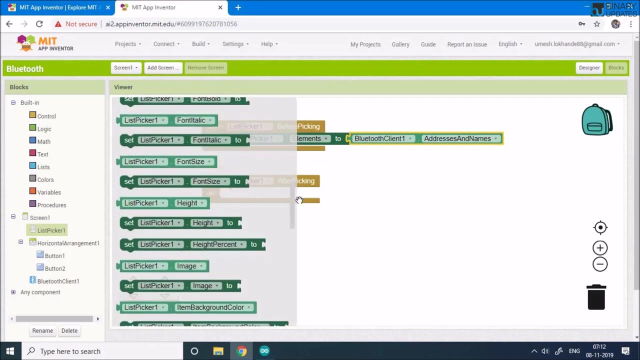 list of elements, right, and i would select a bluetooth client address name, basically, and i will put it here: right. so that's how it works. and then we have to go to this speaker once again and then we have to take the selection okay element and the selection. so where is it? let me look in it. 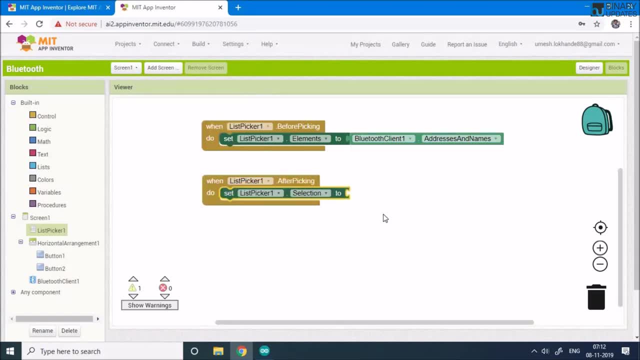 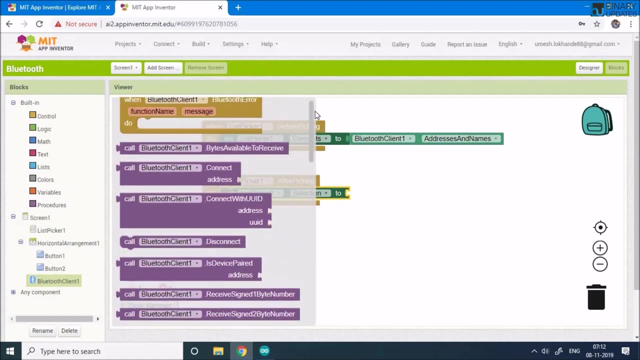 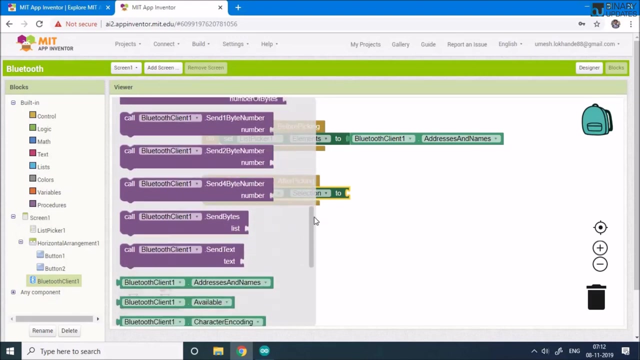 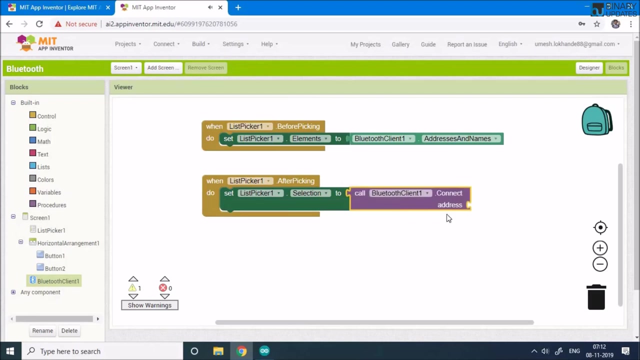 okay, so here's that component we are looking for, and then I need to go to the Bluetooth element and then we have to select for the Bluetooth client and the Bluetooth client is to connect. so okay, this one we won. because whenever we press the, whenever we press the, 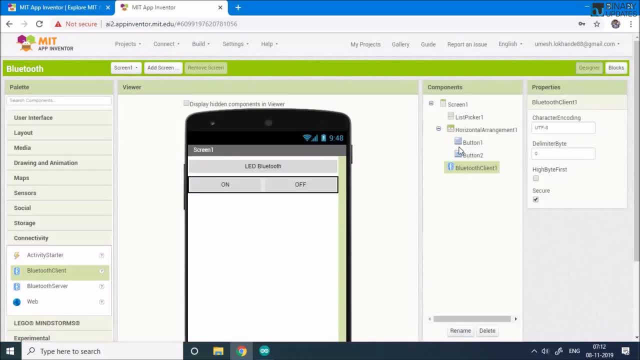 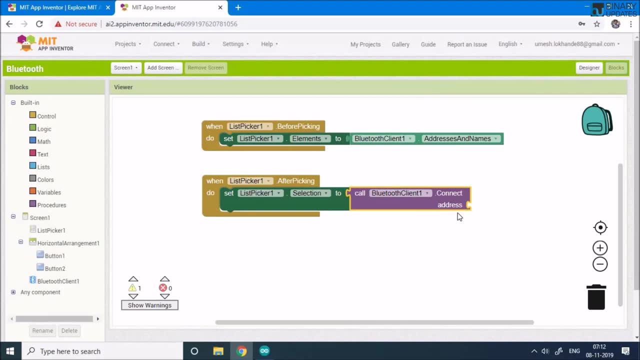 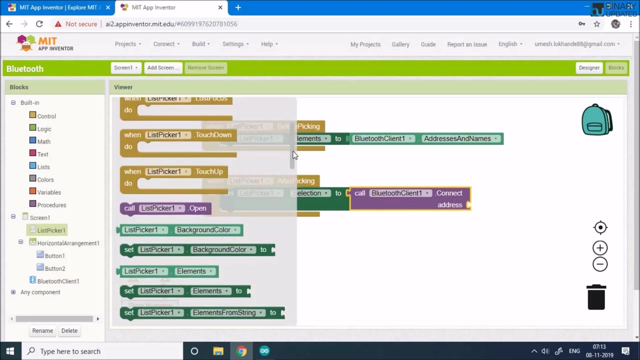 list speaker, one that means LED Bluetooth button. this button- okay, this button- then it will give us the list of Bluetooth connected Bluetooth client which are paired with your mobile phone right on which this app is running, basically. so the next component is a list speaker, and then we have to select. 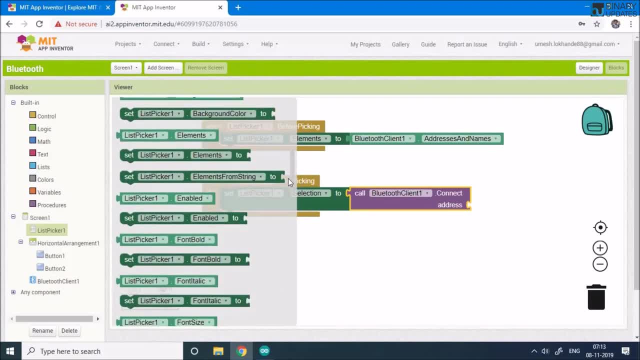 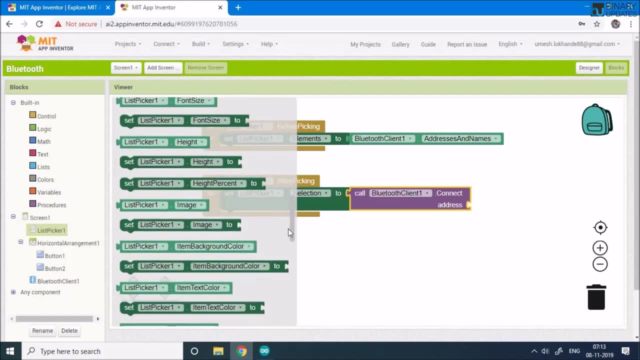 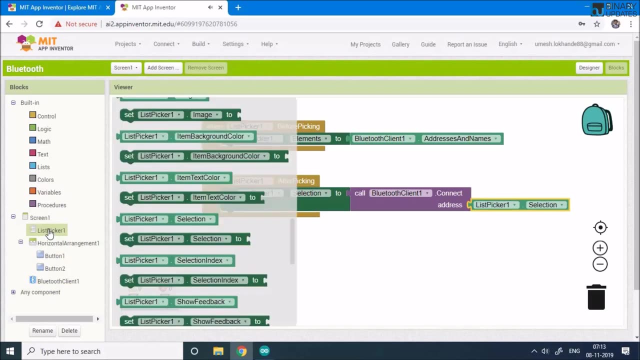 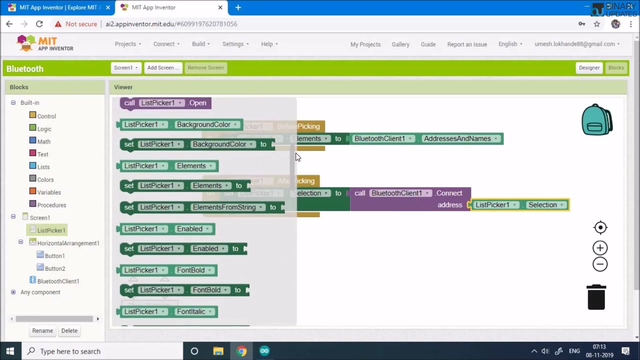 the list speaker: one selection element. this speaker: one selection element. so this is that one we are looking for, and then we have to go to this speaker once again and we just want to throw the text right. so whenever you select the HC 05 Bluetooth module, then the button name: 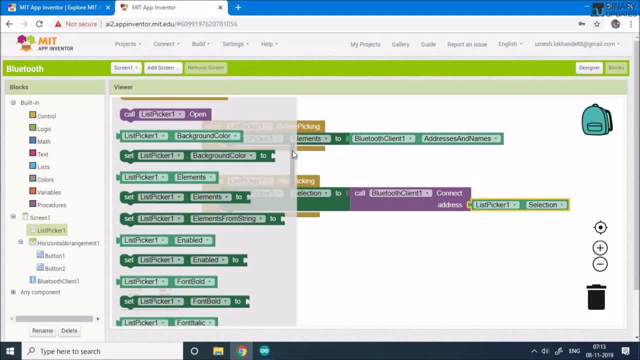 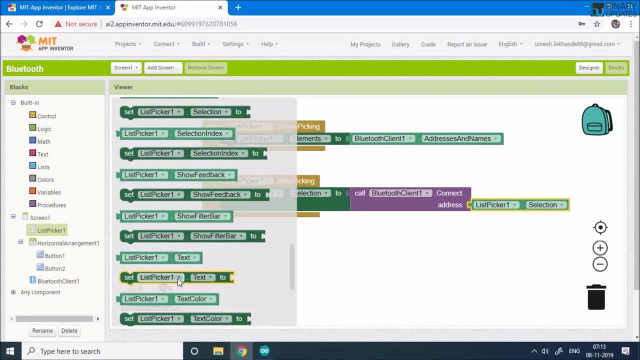 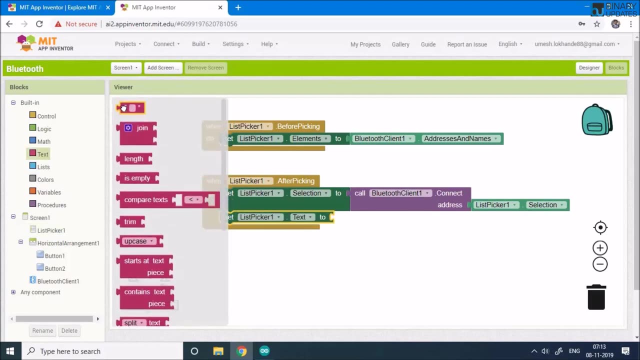 has to be changed from LED Bluetooth to say, for example, something like connected or something right, so it will make a little more sense. so I will take this one and put it here and then go to text and then just add a normal text. so whenever you select the Bluetooth client, then okay, it will change the text to be: 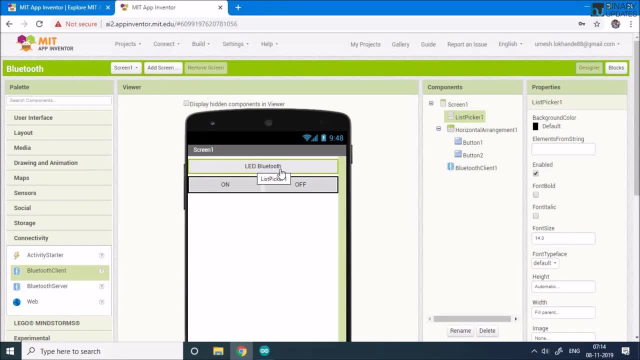 connected. so once you press the button in order to connect to the Bluetooth Arduino Bluetooth. when you press this button, then it will give you the list you select, that's the 05, and then the name of this button will be changed as a connected. so you then confirm that your mobile phone and the 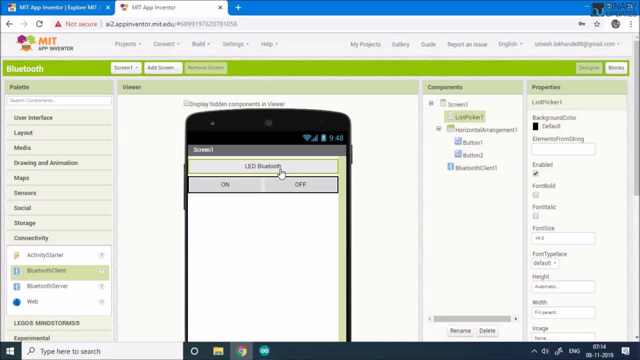 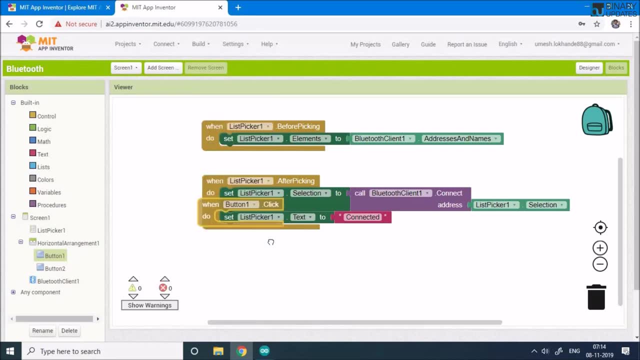 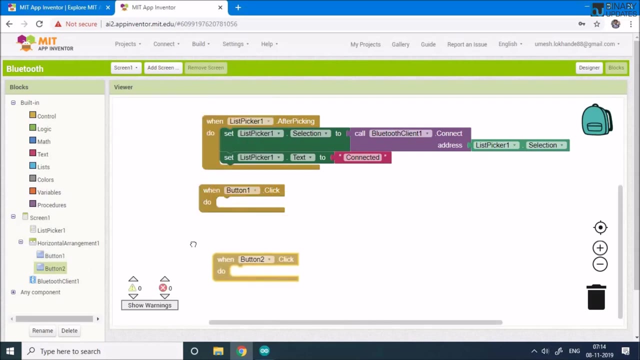 app is connected to your HC 05 Bluetooth module, which is connected to Arduino, then go back to the blog section and in a button I have to take button one and then we have to go to button two and take the button two, right, so here we have two buttons, okay, and then we have to write a logic where, when we 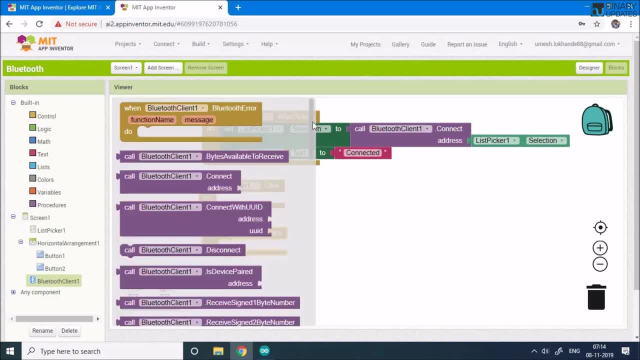 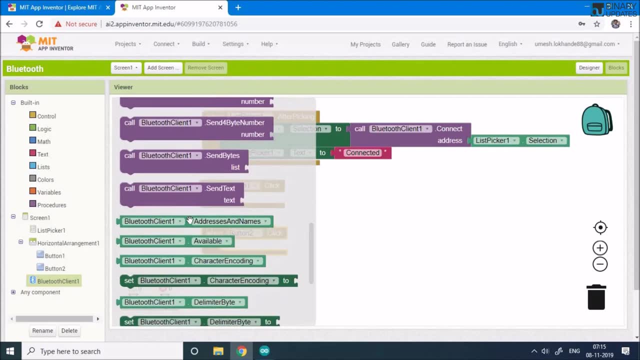 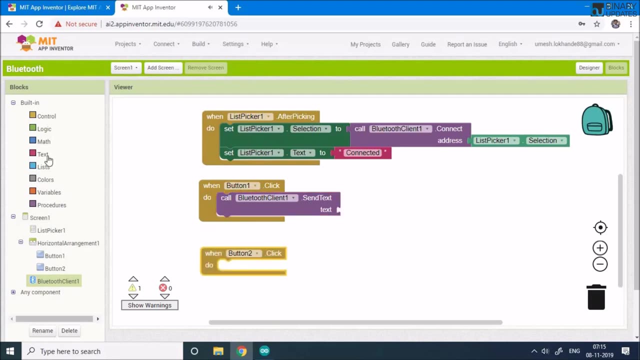 press the button one, then the button one will send the text to Arduino over at c05, right? so this will be a send text element that we want to put here and then in the text section we want to. so whenever somebody press the button one, then it will send one, so that will turn on the LED connected to Arduino and then 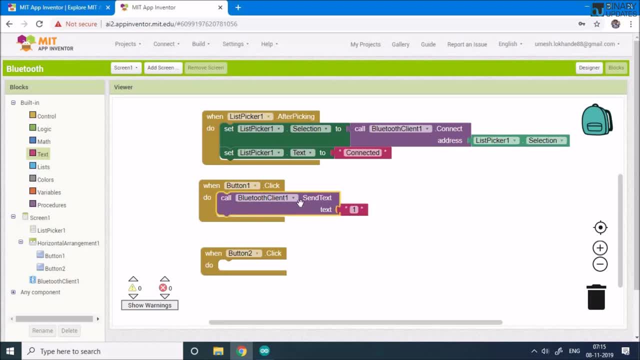 you can copy and paste, by the way, so I can just duplicate the element and put it here and I would just say zero. so whenever somebody press the button two, it will send a zero, right, accordingly. our logic is written. so when we press on button, then it will send. 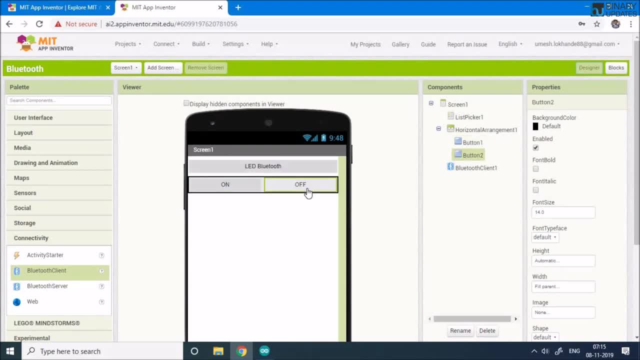 one, because that's what we wrote. and when we press off button it will send zero, so it will turn off the led connected to arduino right. so on button will send one and turn on the led. when you press your button it will send zero to arduino over bluetooth module and it will turn. 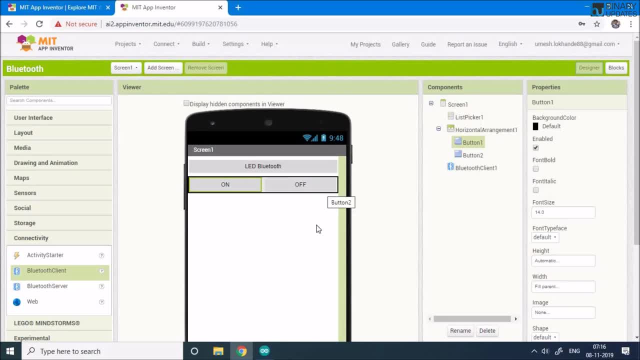 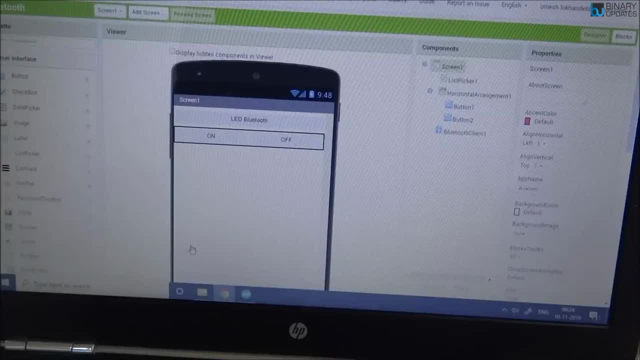 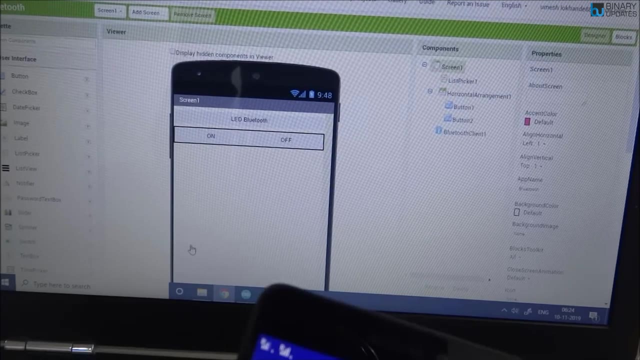 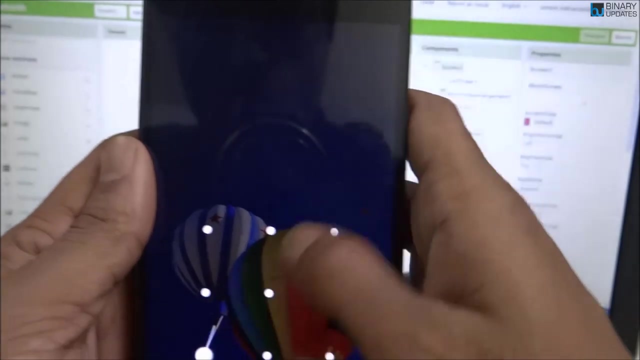 off the led. that's how you create, basically in mobile app, using mit app inventor. now to make this app work with your mobile phones. now, once the project is ready on a screen, then we have to take our phone in order to transfer the mobile app from our mit app inventor to the mobile phone. so let me take my mobile phone on. 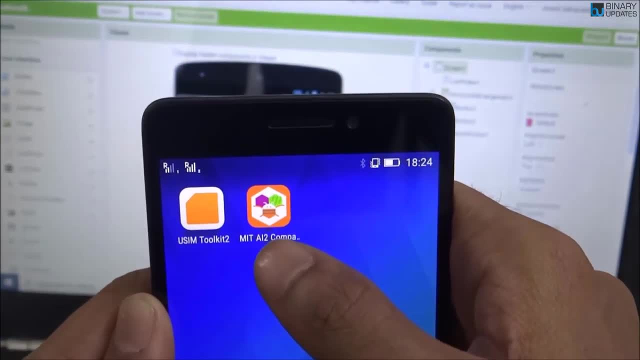 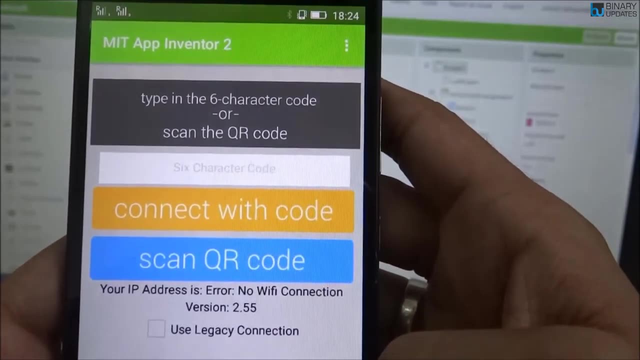 okay, and then i would open up this mit ai2 companion app. okay, and then you see no wi-fi, so continue without wi-fi, that's fine. and then i would go here, okay, and then i would go here, and then i would go here, and then i would go here, and then i would. 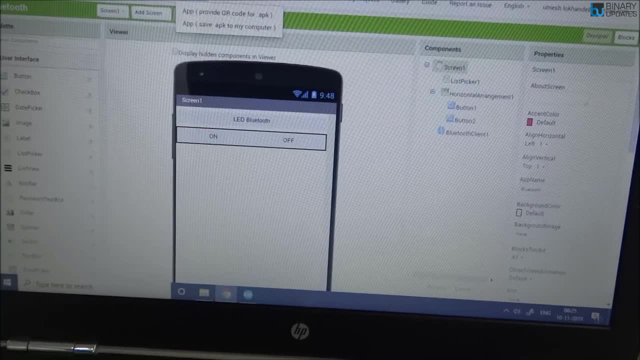 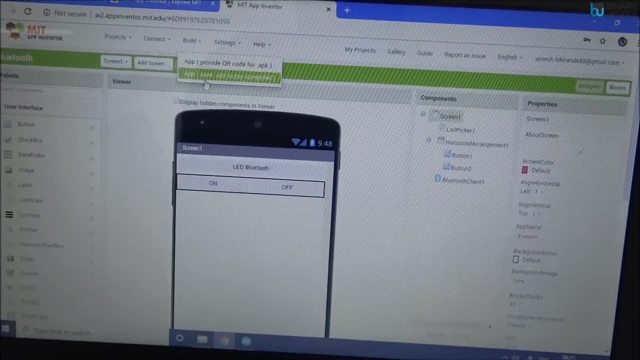 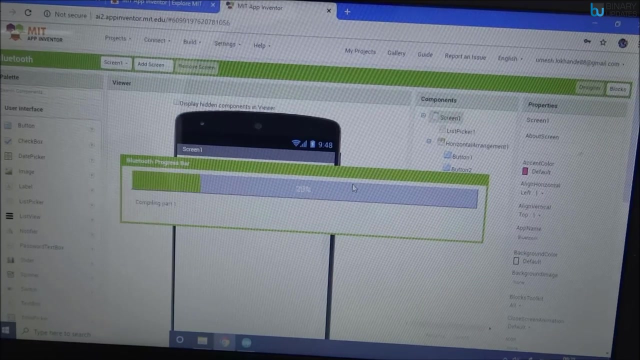 in the build. i will select the build option. i hope you can see. let me just turn on. so here's the build option. i can select: provide a qr code for apk, and in a moment there will be and qr code will be generated. if not, maybe then we have to turn on the wi-fi, but i don't think its. 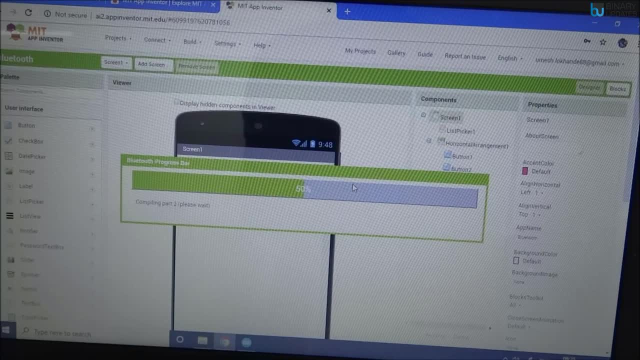 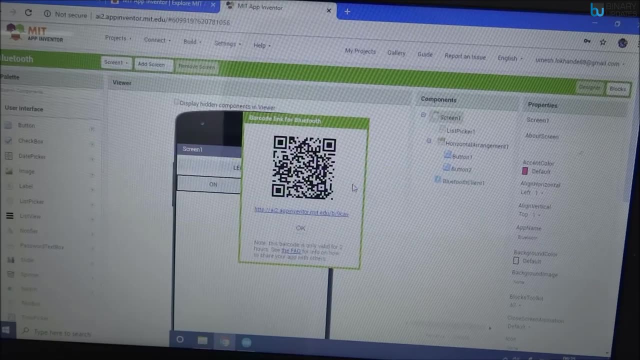 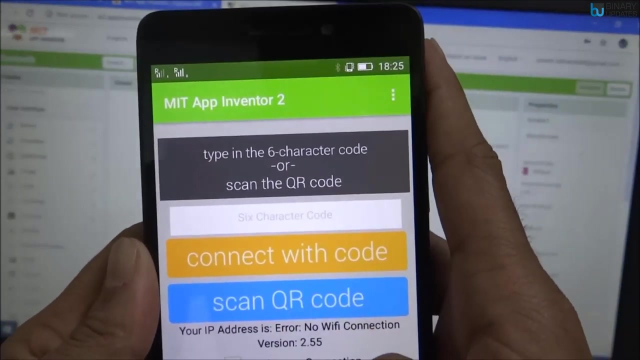 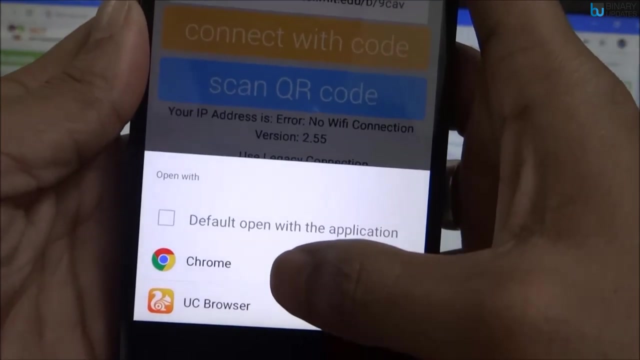 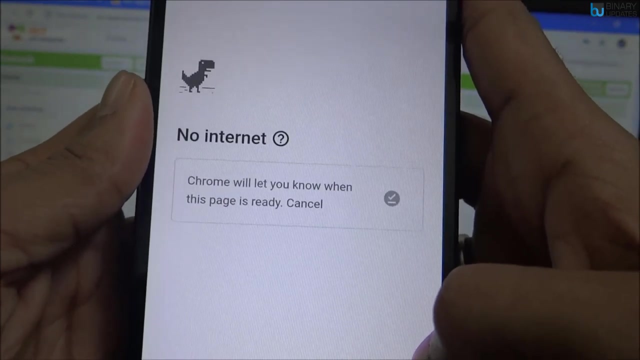 needed. let's see what happens. so we see the QR code is there so I can take my phone and connect scan QR code. I can click on scan QR code and here is the QR code I can scan and I will click on Chrome here and it will start installing this mobile app. right, I hope. 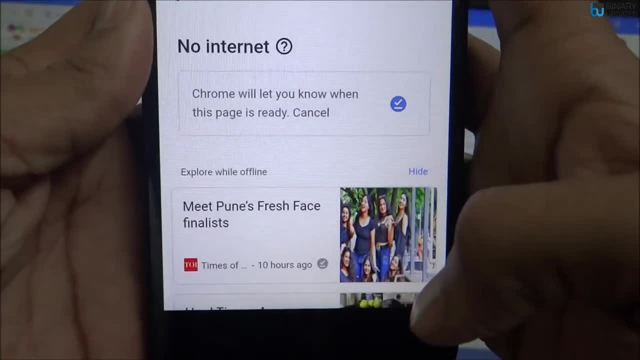 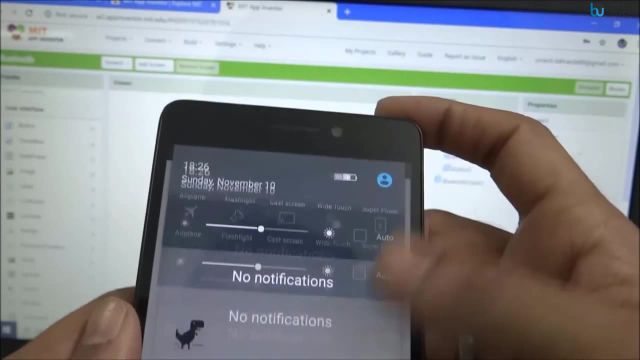 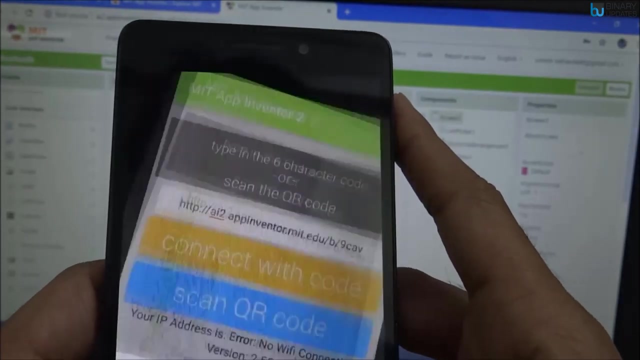 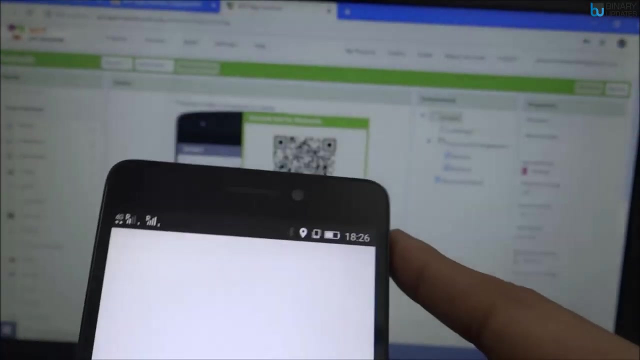 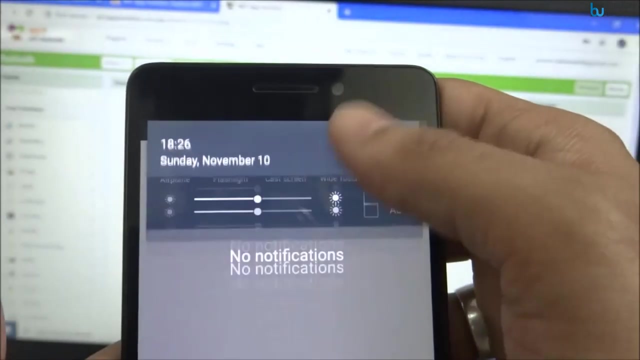 so it will come up. oh no, there's no internet, so I have to turn on the data network here. okay, and just try once again. okay, so scan QR code, and here I scan again. okay, and then select the Chrome and then you see: oh no, this is what's up. okay, it says: 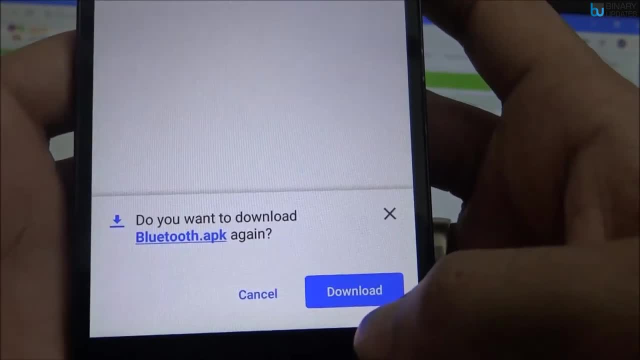 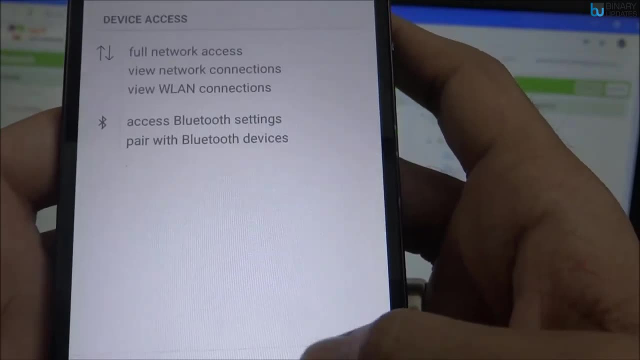 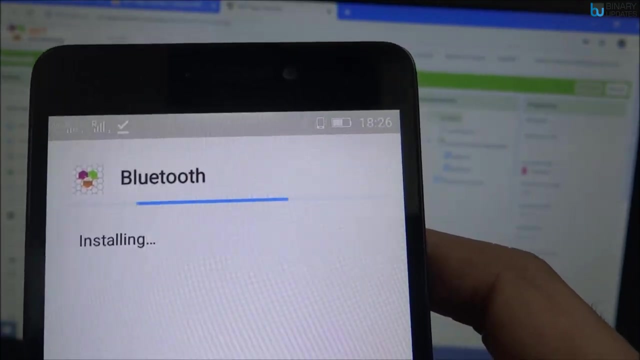 in the down corner. do you want to download? yes, I want to download. so let me press the download button and you see, now app is installed. I can say open, install and it is installing right. okay, it's very easy. you don't even need to create, generate an APK. it can transfer. 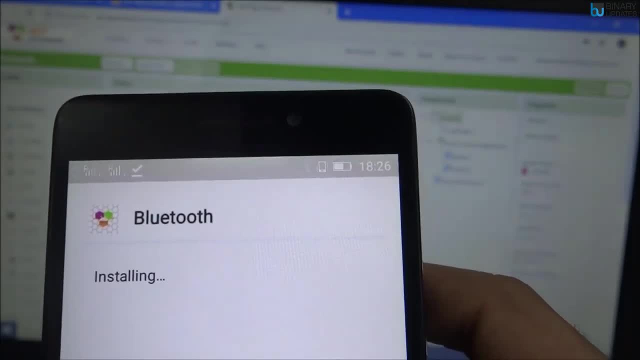 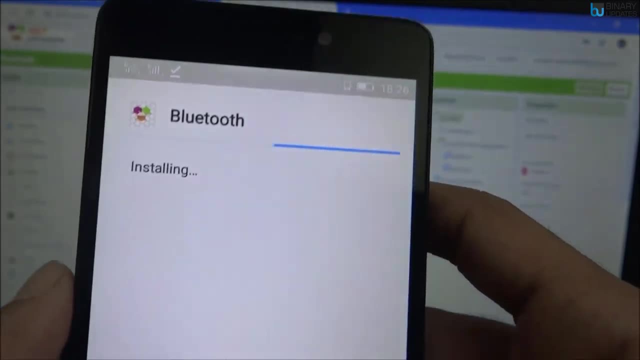 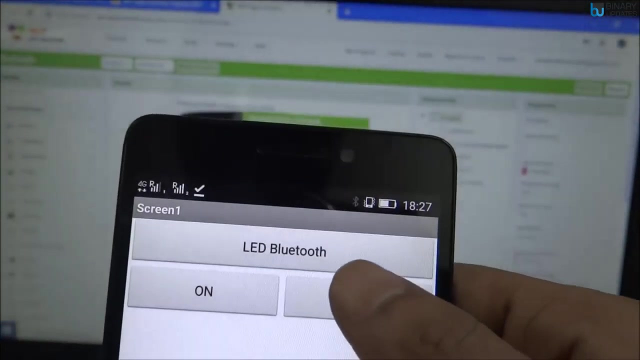 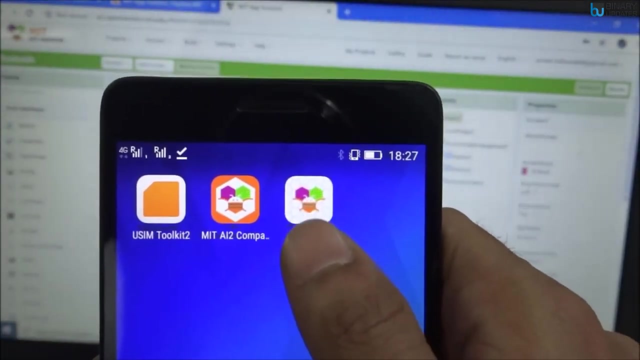 the APK from the app inventor straight away to your mobile phone. okay, app is installed and I can say here, open button and here is my app. I can now use this app later. right, so this is how the shortcut looks like for the Bluetooth app that we have installed. so I can now use this app later. right, so this is how the shortcut looks like for the Bluetooth app. 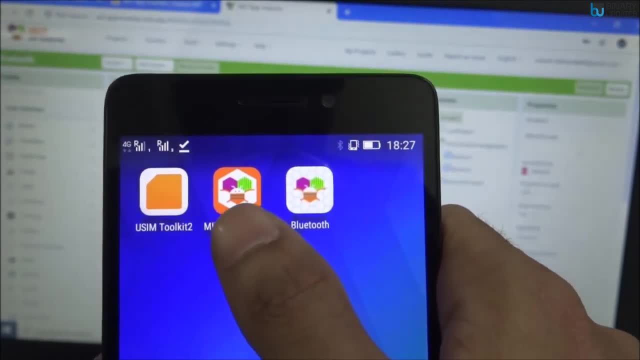 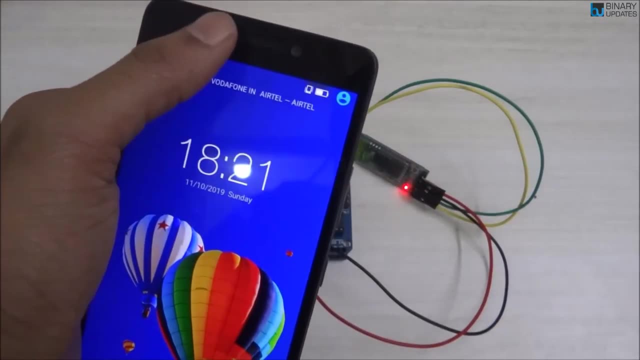 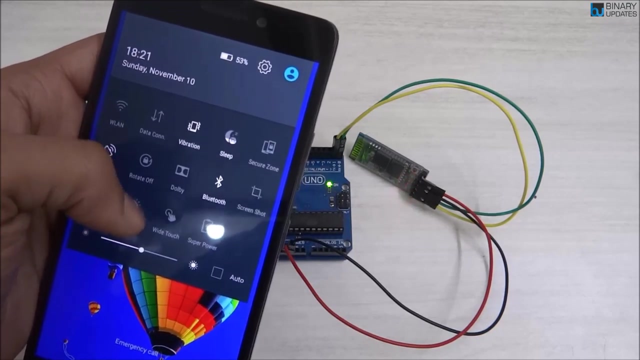 that we have created, and this is MIT AI 2 companion app. right, you need to download this first before you use it. right, we have to take our mobile phones. okay, and because we are using Bluetooth as a protocol, we have to turn on the Bluetooth first on our phone. once the Bluetooth turns on, you see the phone. 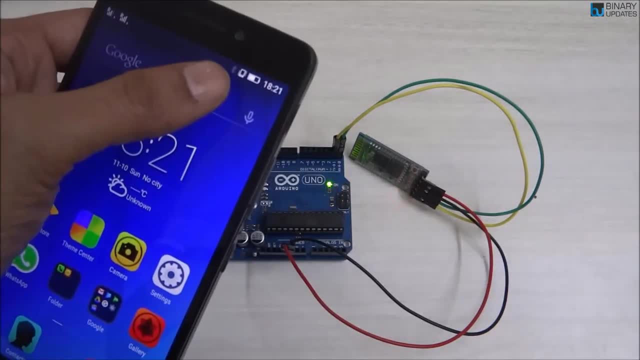 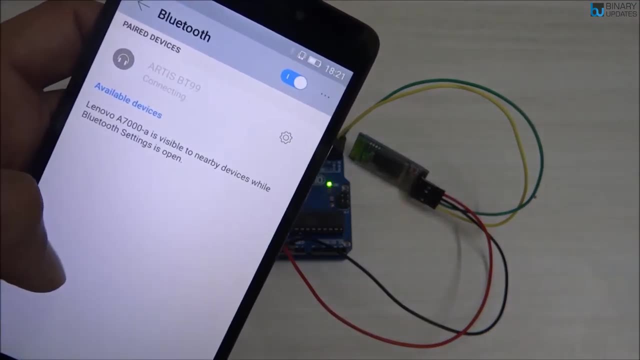 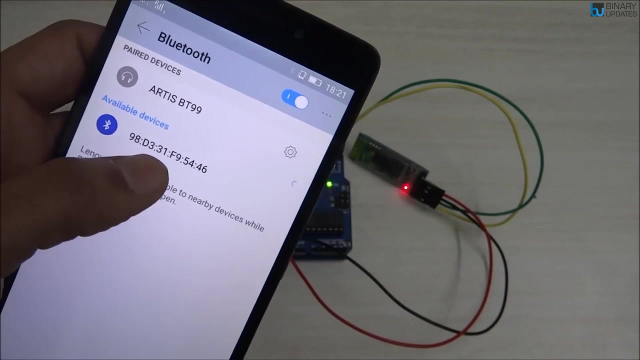 will show you the Bluetooth is on right. once the Bluetooth is on we go to settings on phone and then inside the Bluetooth option, you will see it will list the client which is available, right? so 983 is one of the Bluetooth client and you see, my load module is powered up so I can able to see it. so let me.